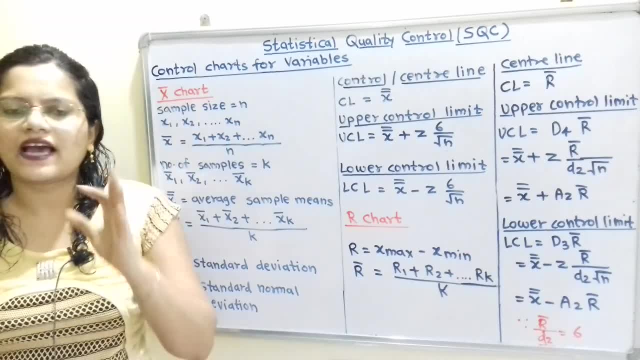 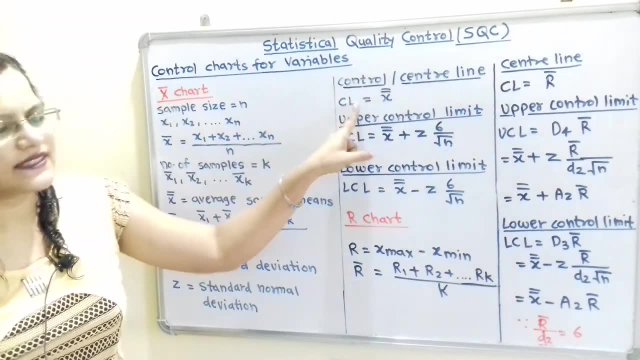 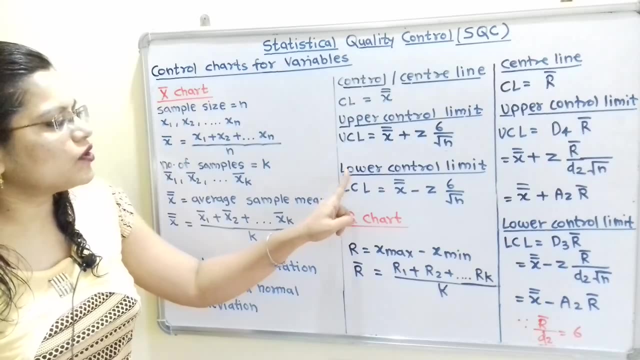 Now, to draw this X bar chart, there are three parameters required. First, one control or center line, which is known as CL. Second, one upper control limit, that is U. Second, one upper control limit, that is U. And third, one lower control limit, that is LCL. 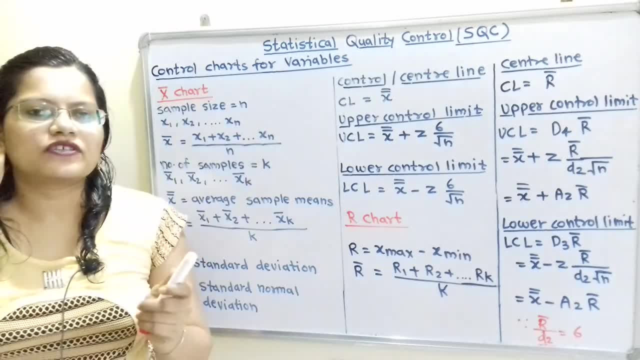 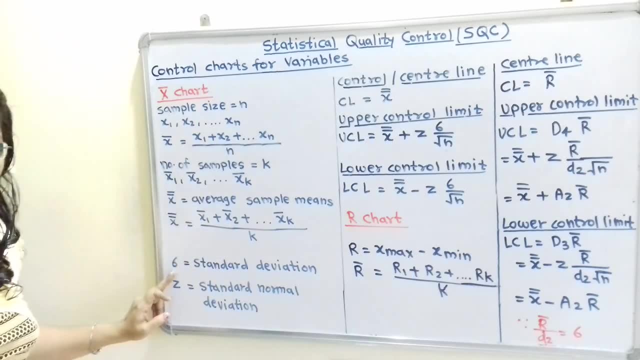 So these are the three important parameters to draw the X bar chart. So for that we will use the two notations: First one sigma, that is the standard deviation and that is mentioned in the question. Then Z, that is standard normal deviation. So this value of Z is mentioned in the question. 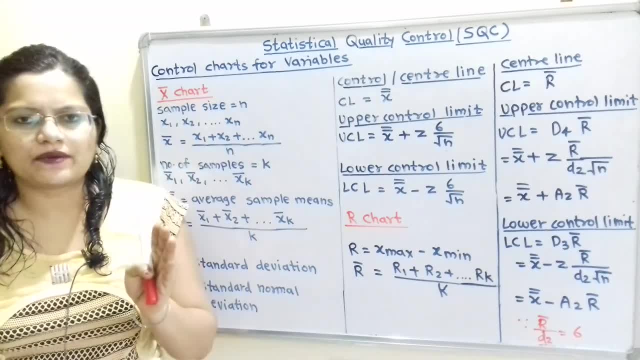 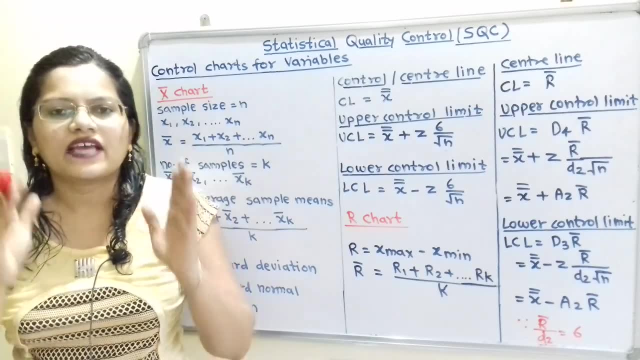 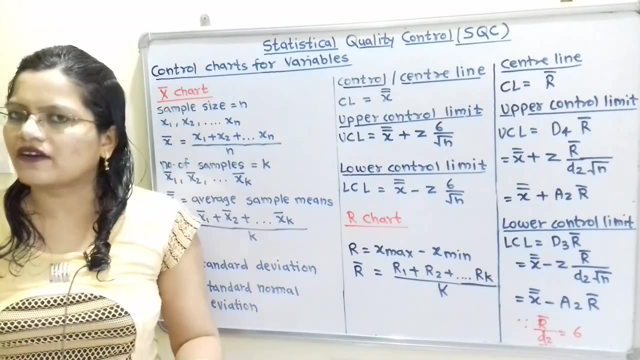 In such a way that that is, there is two sigma or three sigma. So suppose there is two sigma- that word is mentioned in the question, then value of Z, we have to consider two. Suppose there is three sigma, that is mentioned in the question, then value of Z, that is standard normal deviation, we have to consider as a three. 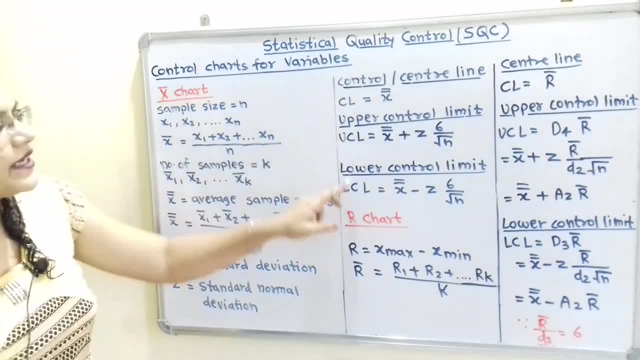 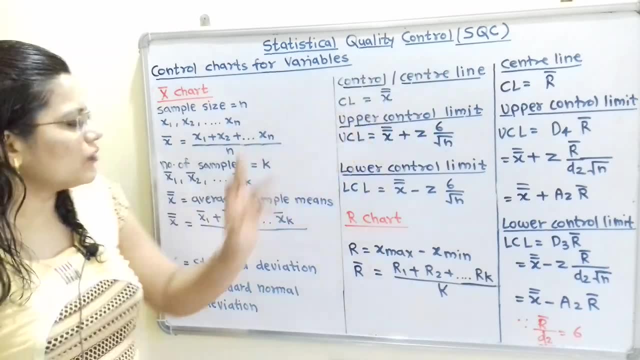 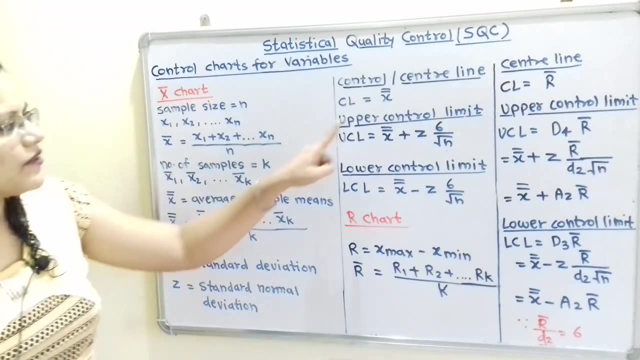 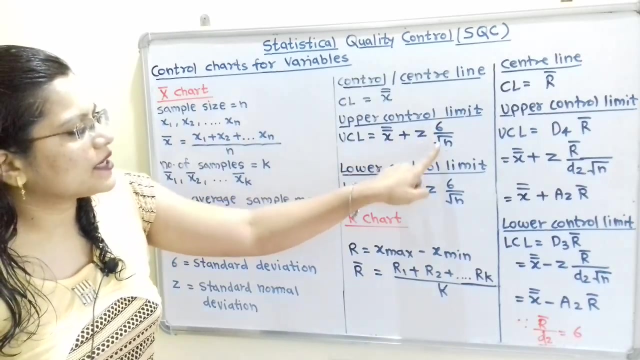 Now we will move how to calculate these three important parameters. So center line, that is CL, and we will take this value as X double bar. So X double bar can be calculated by using this formula. Then second, one upper control limit, that is UCL, which is equal to X double bar plus Z sigma by root N. 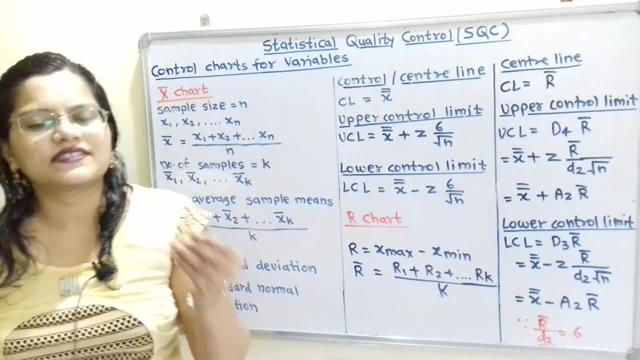 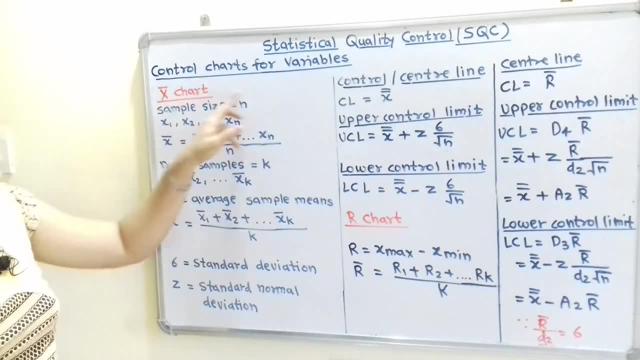 So this sigma is also mentioned in the question. that is the standard deviation and this root N, that is N is the number, Number of samples, that is the sample size In each sample. number of readings or number of units are there, and that is the value of N that we have to consider here. 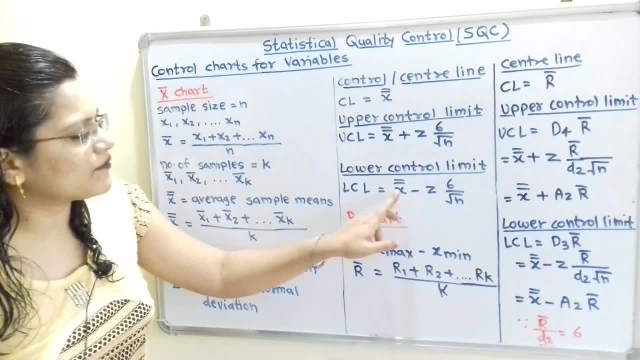 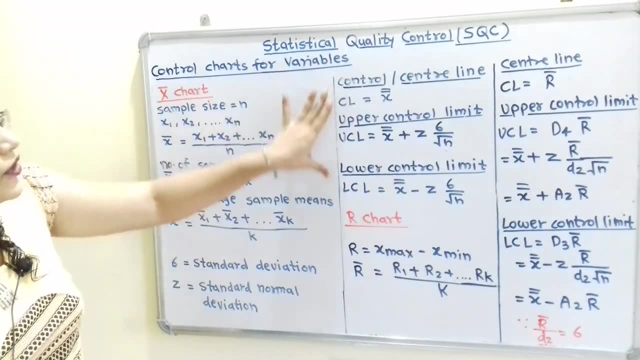 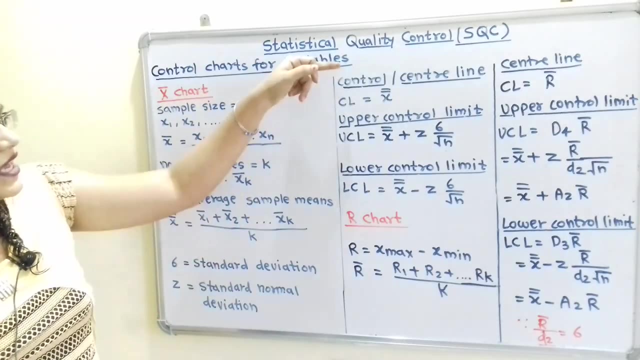 Now for lower control limit. LCL is equal to X double bar minus Z into sigma by root N. So if we observe, these three parameters are required to draw the X bar chart. So with the help of all These three we can easily draw this X bar chart. 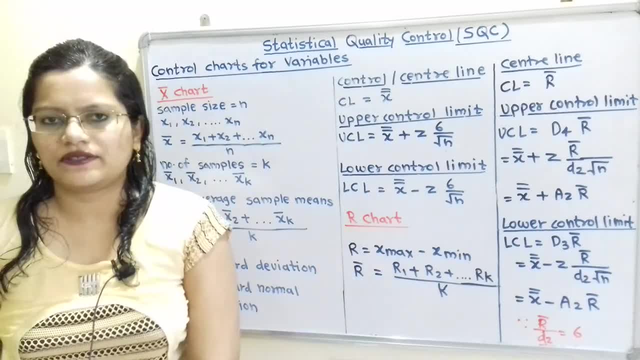 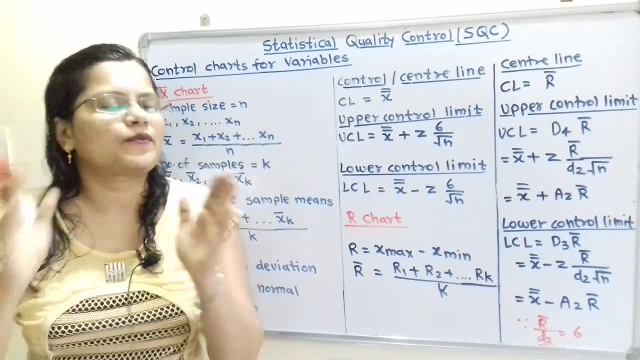 Now we will move to the next point, that is the R chart. So for this R, that is the range. So how to calculate this range? So for each sample, suppose there are N number of readings, that is, X1,, X2, up to XL. 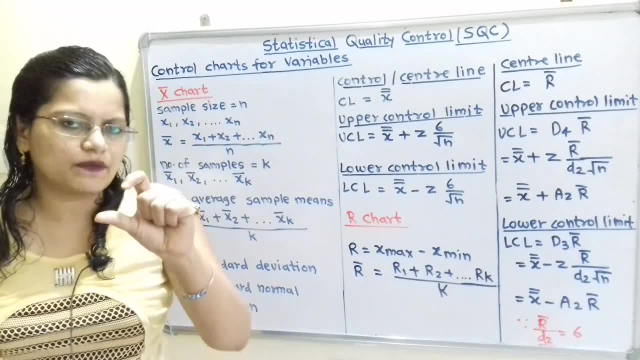 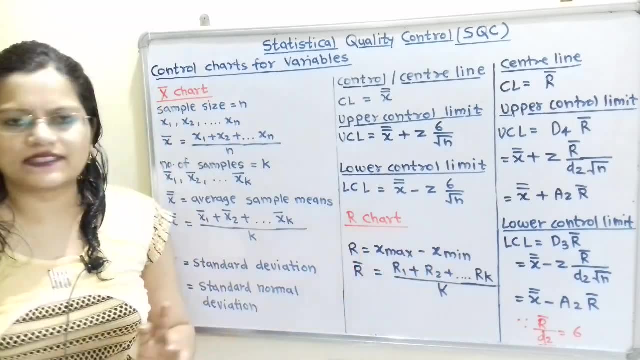 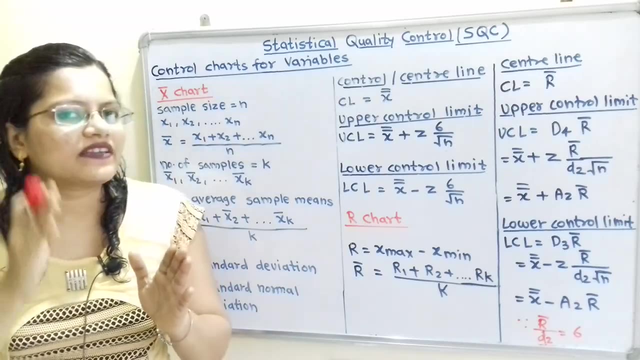 Then out of these readings we have to find out the maximum value and minimum value And the difference in between this maximum and minimum is more, So it is easy for us to calculate range for each sample. So for sample 1, range is R1.. 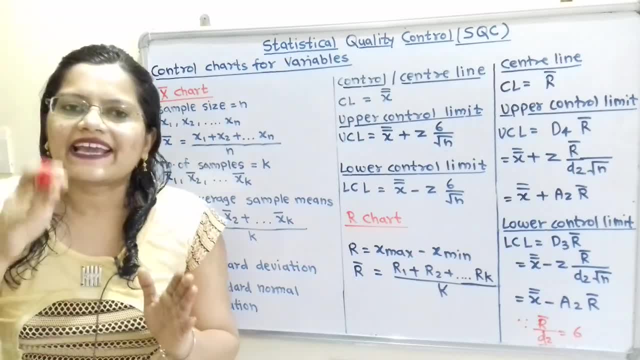 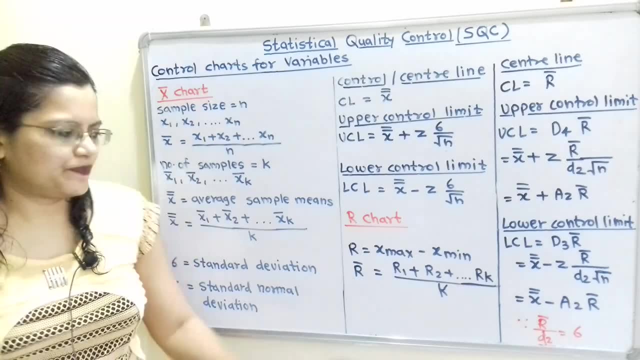 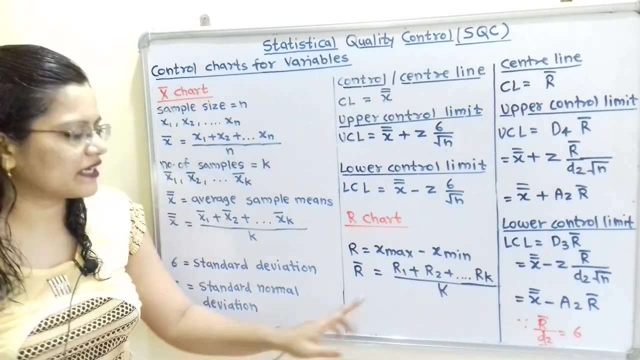 For sample 2, range is R2.. And for the kth sample, because number of samples, k, that is the range, is known as R3.. So R is equal to X maximum minus X minimum and R bar is equal to: that is the average. 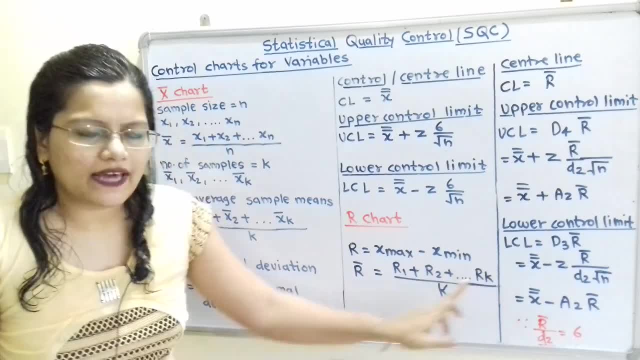 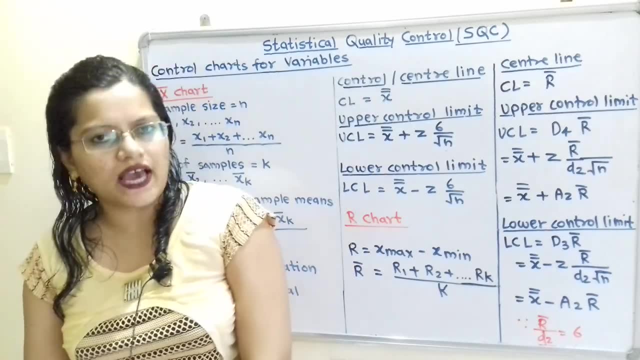 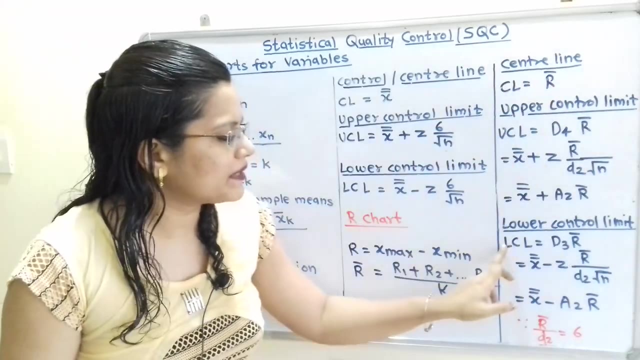 That is equal to R1 plus R2 plus up to R3.. So that is equal to Rk divided by k. Now again for this R chart also, three parameters are important. First one center line: CL. upper control limit: UCL. lower control limit: LCL. 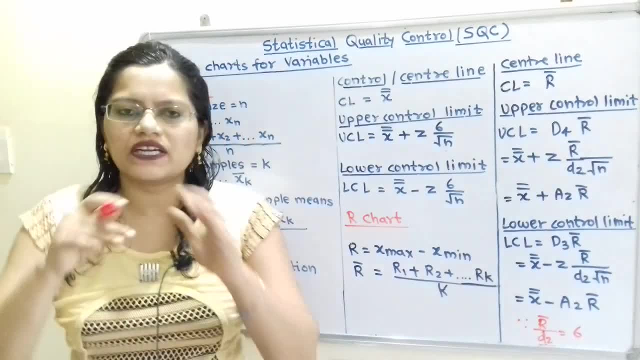 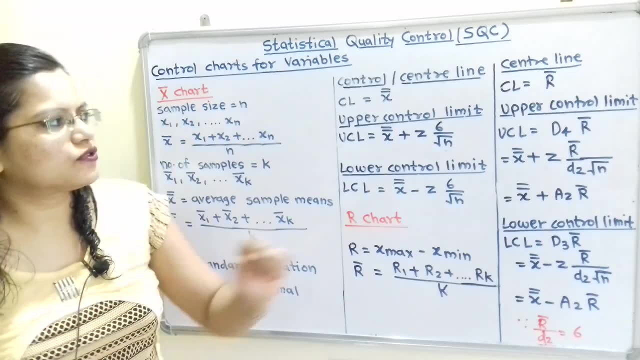 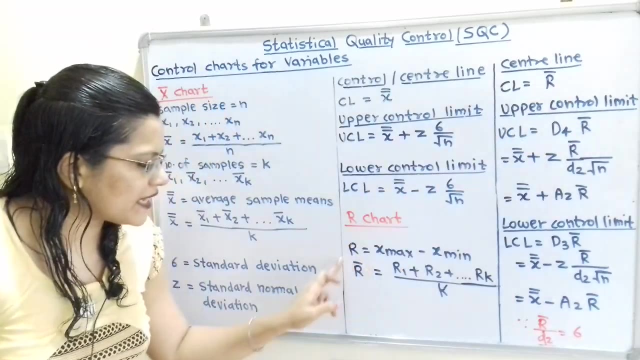 Now there are the different values that are mentioned in the chart, and that chart is provided in the examination. So which are those values? So now, this center line, That is CL, that is equal to R bar and R bar we can calculate by using this formula. 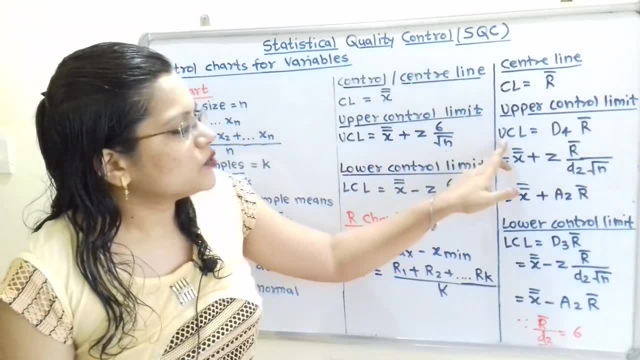 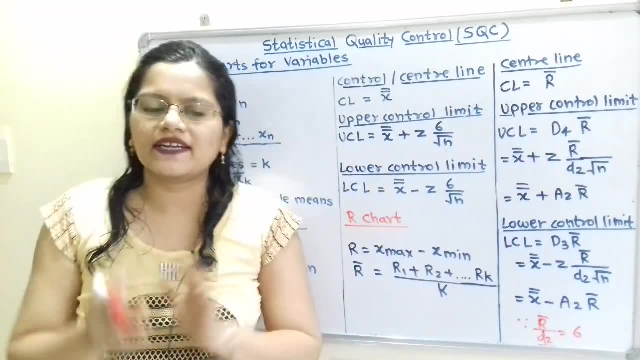 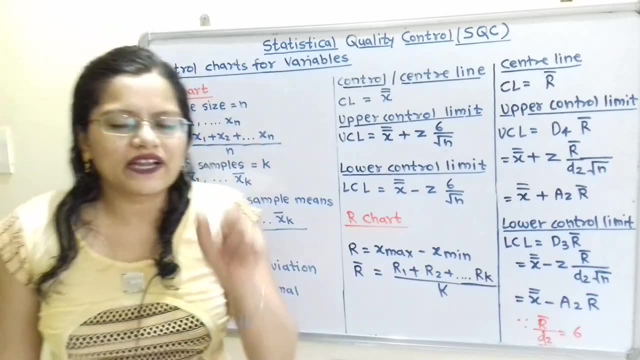 Now for the upper control limit, UCL default R bar. Now this value of default that will get from the chart provided in the examination and that will depend upon the value of N, So we have to refer this sample size N And for this particular sample size N, 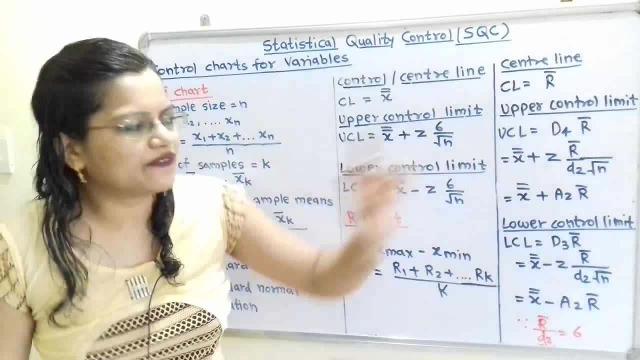 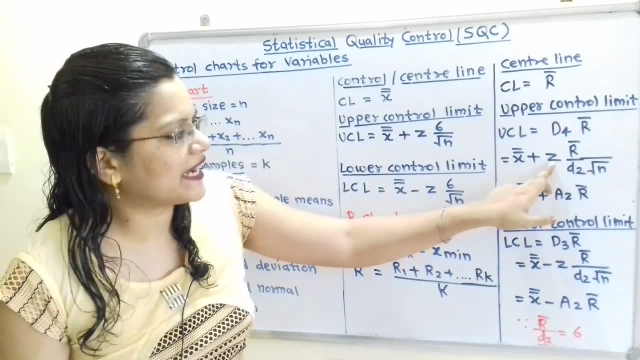 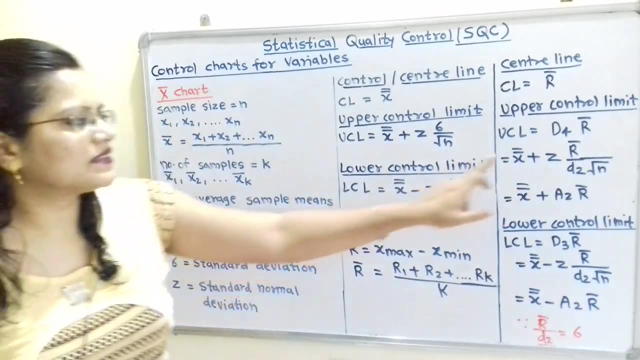 So we have to refer this sample size N, We have to take the value of default. Then again, which is equal to. we can use this second formula: X double bar plus Z R bar by D2 under root N. So here X double bar that we can calculate Z. that is mentioned in the question. standard normal radiation. 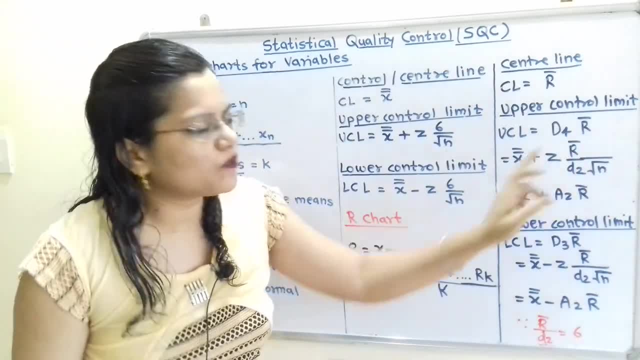 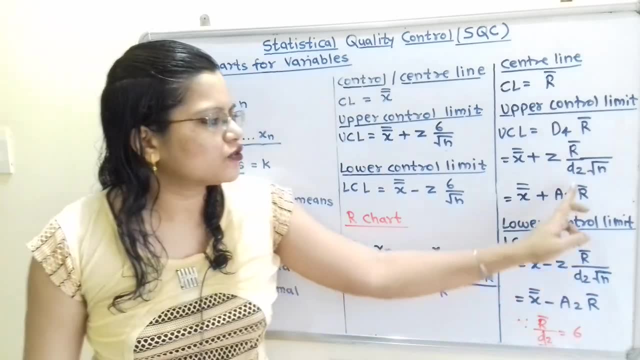 R bar that we can calculate. And what is this small D2.. So this D2 also mentioned in that chart. So this D2 also mentioned in that chart. So this D2 also mentioned in that chart. So this D2 also depends upon the sample size N. 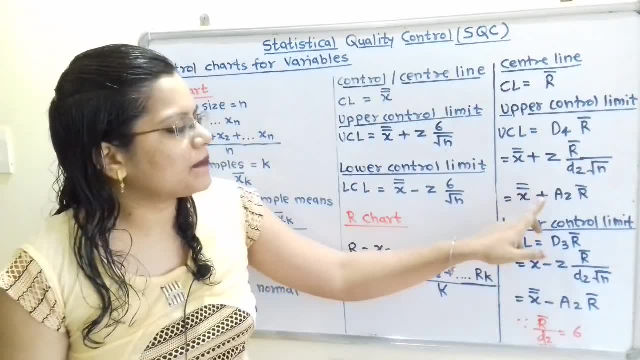 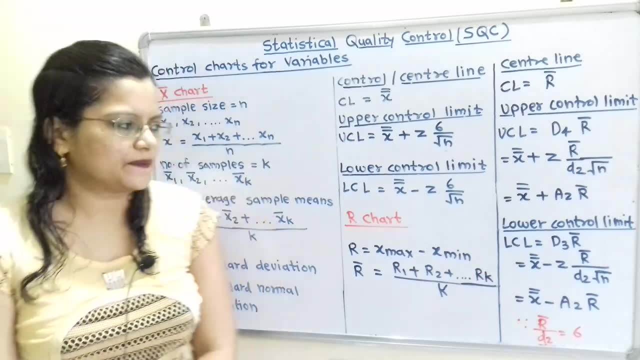 And here under root of N is the sample size. Then the next formula is X double bar plus A2 R bar. So this value of A2 is also mentioned in this control chart. Then the lower control limit. So for this lower control limit, 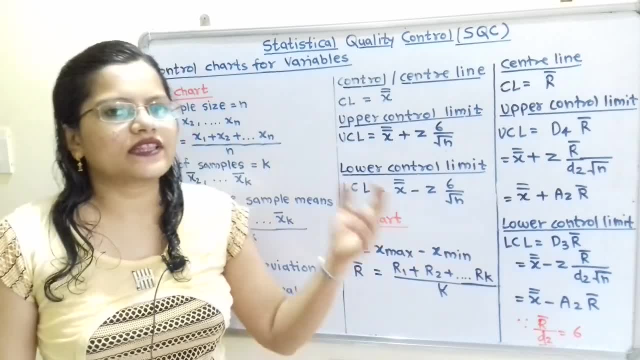 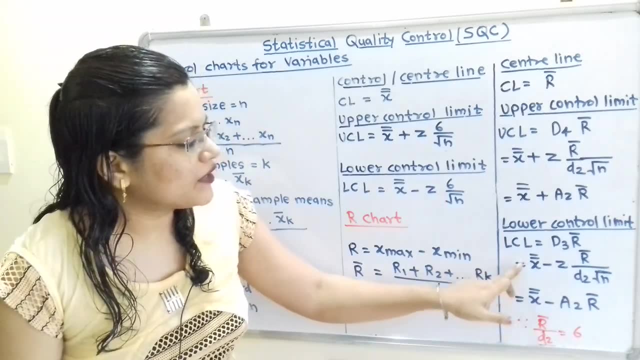 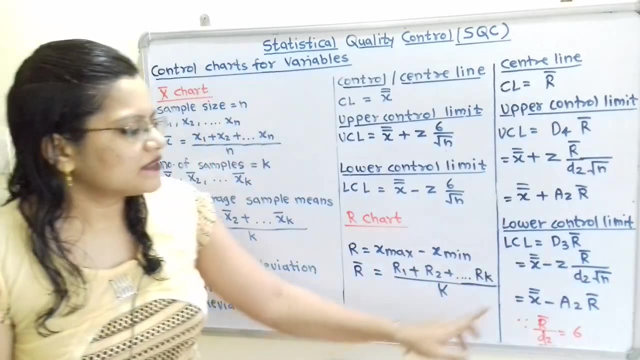 Then CL is equal to D3 R bar. D3 depends upon the sample size N, And that is the value of A2.. n and that is the chart provided in the exam, which is equal to so, second formula: x double bar minus z r bar by d2 under root of n. and the third formula x double bar minus a2 r. 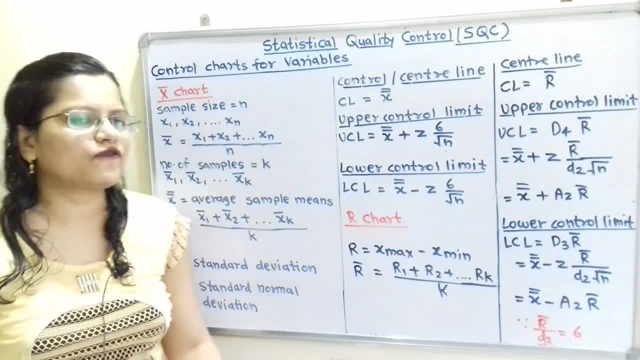 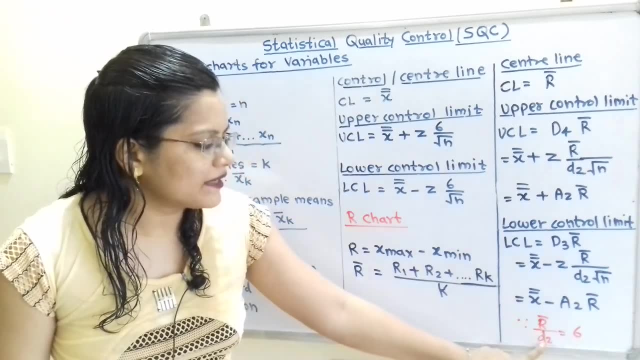 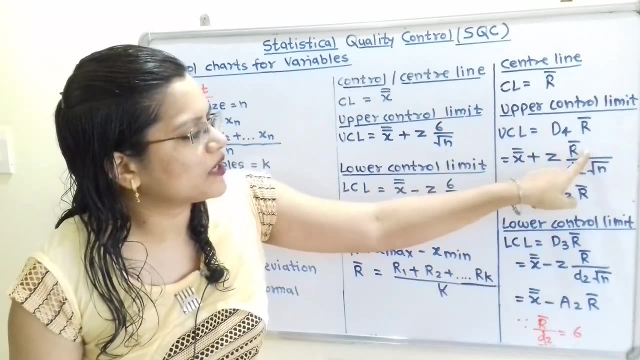 bar. so here value of a2 and d2. we can find out from this sample size n, and we can also say that sigma is equal to r bar by d2. so we can calculate the sigma, because here instead of r bar by d2 we can use the formula that is sigma by root n. so here all these formulas. 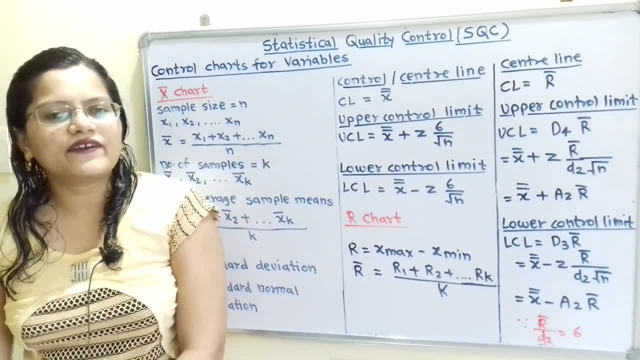 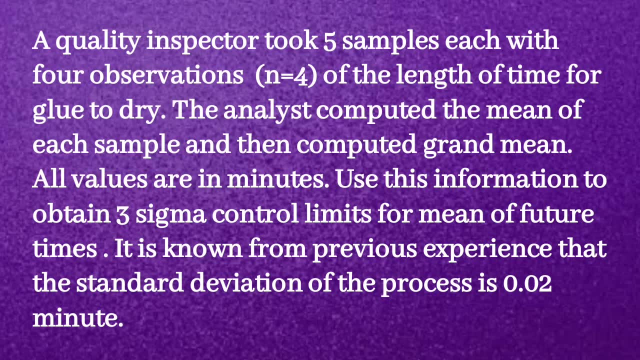 you have to note down in your notebook and which is important to solve the problem. given question: a quality inspector took 5 samples, each with 4 observations. given question: a quality inspector took 5 samples, each with 4 observations, of the length of time for a glue to dry. the analyst computed the mean of each sample and. 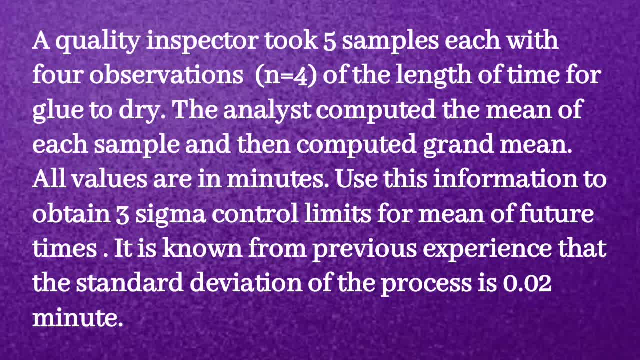 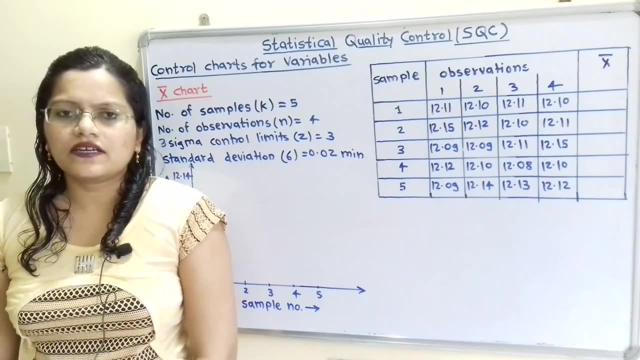 then computed the grand mean. all values are in minutes. use this information to obtain 3 sigma control limits for mean of future times. it is known from previous experience that the standard deviation of the process is 0.02 minute. let us understand the given data mentioned. 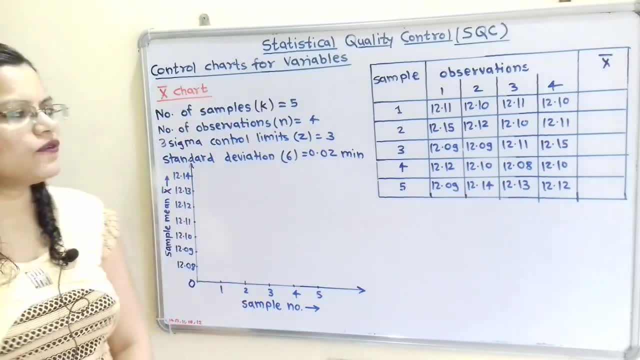 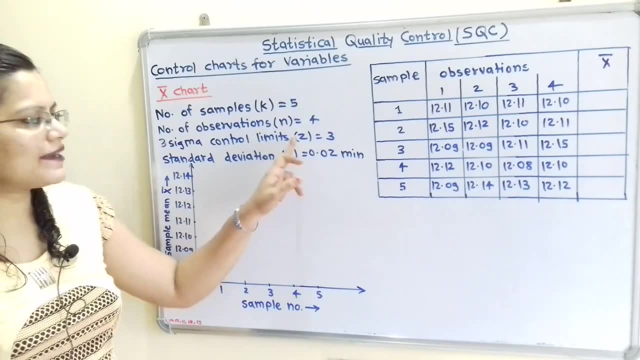 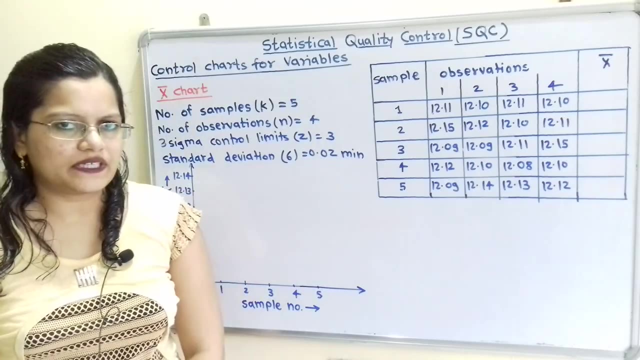 in the question. number of samples k is equal to 5, then the number of observations n is equal to 4. 3 sigma control limits. that means z is equal to 4 and standard deviation sigma is equal to 0.02 minute. now in question this table. is mentioned, that is, for each sample. KQ and Z is equal to 9 ДFs and Ds. the total день üq unit value and mass data is three: 19913 L ZZ. depth difference. Z equals to task data, joining default equals to target variation and Z equal to dividend. soient In question in the next мужчinawajin. 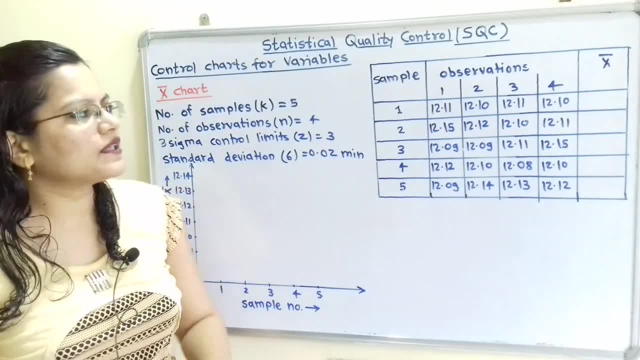 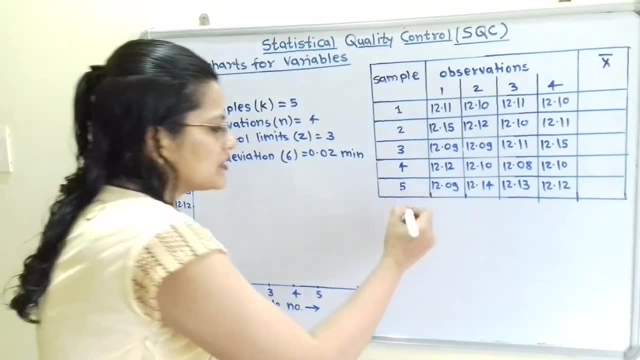 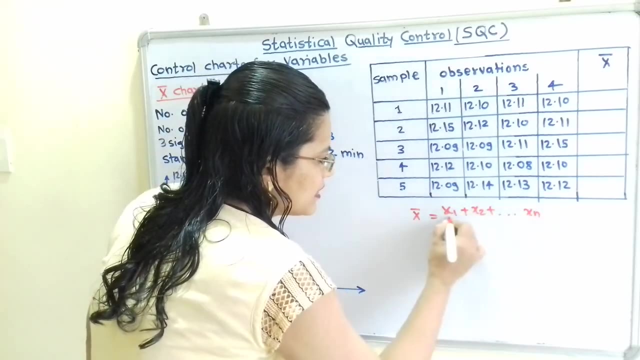 there are four observations. So from this we can calculate the value of x bar. So what is the formula to calculate this x bar? So we have seen that x bar is equal to x1 plus x2 plus up to xn divided by n. Now here n is equal to 4.. So how I can write this? That 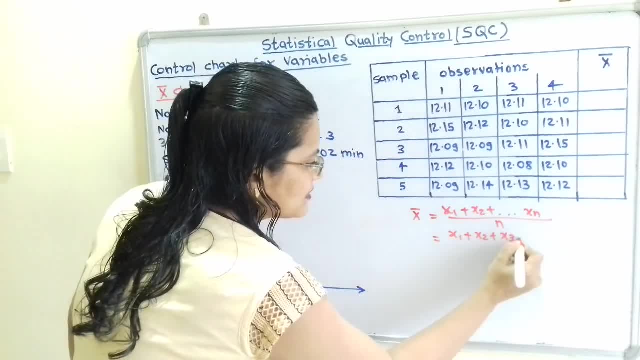 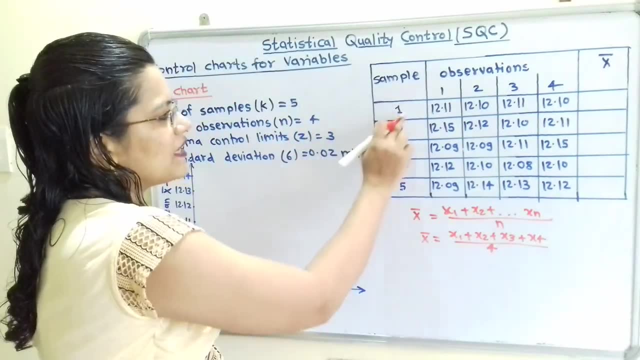 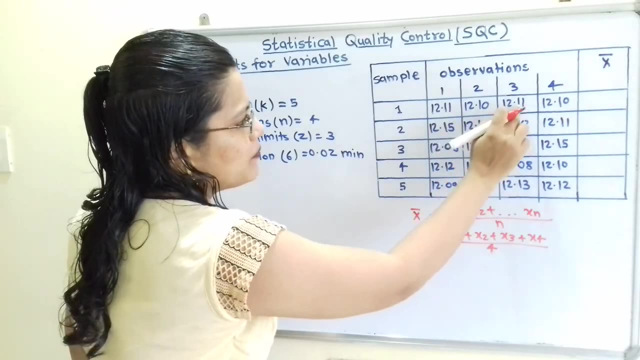 is x1 plus x2 plus x3 plus x4 divided by 4.. So this is the value of x bar for each sample. So that is for the sample number 1, we have to take 12.11 plus 12.10 plus 12.11 plus 12.10. 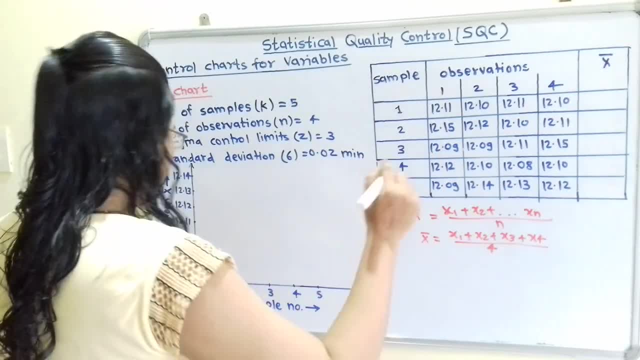 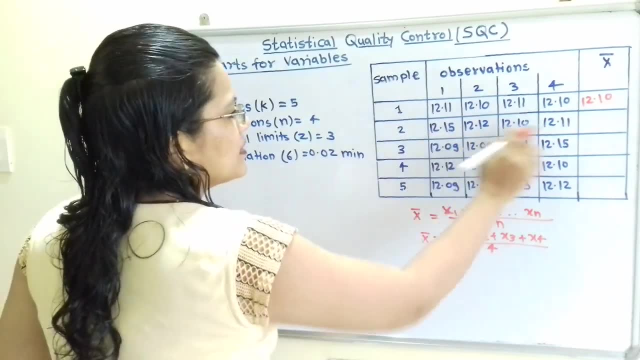 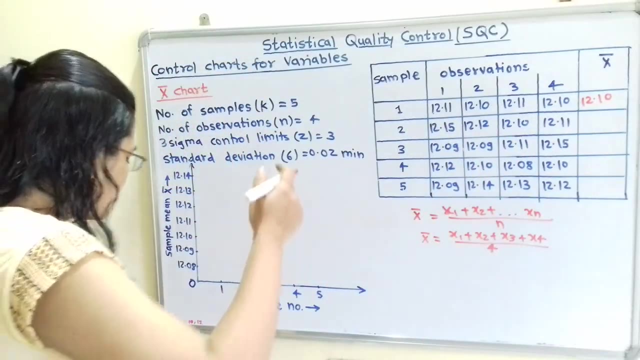 divided by 4.. And this average is 12.10.. Now, in the same way, for this second sample, if we calculate this: 12.15 plus 12.12 plus 12.10 plus 12.11 divided by 4, then it is 12.12. then for the third, it is 12.11. 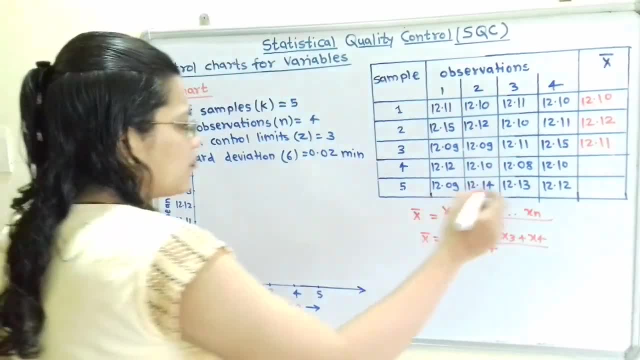 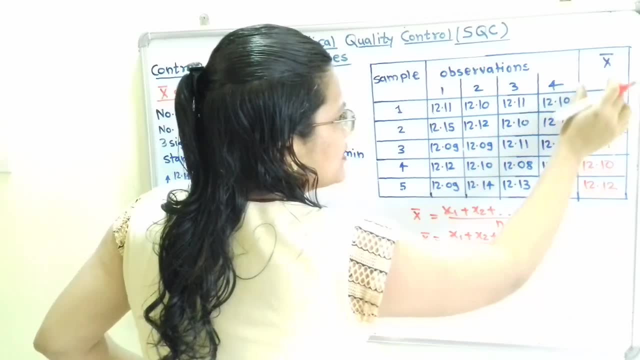 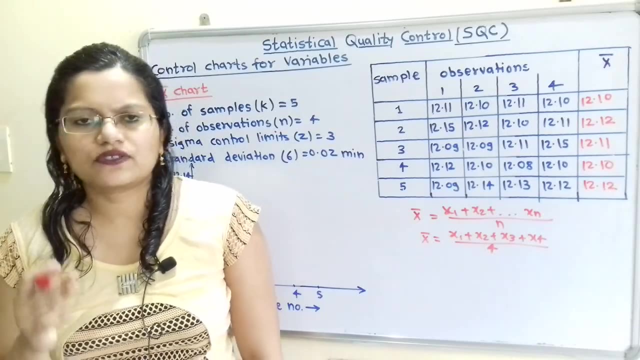 then for the fourth, it is 12.10 and for the last it is 12.12. so this, this is the value of x bar. now we will move to draw the x bar chart. so how to draw this? so for the horizontal line we have: 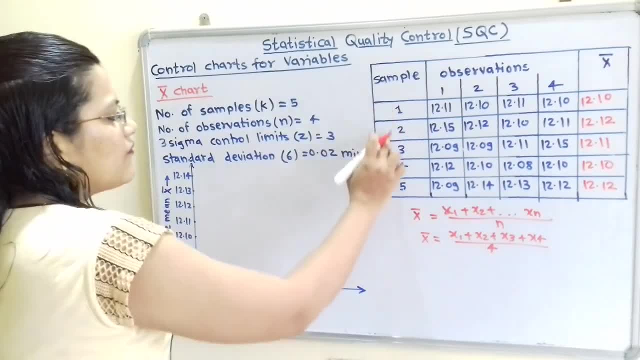 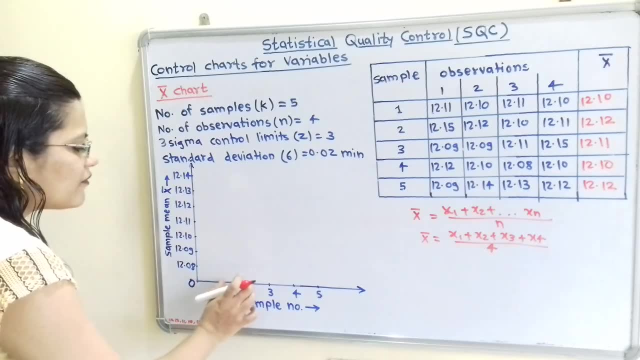 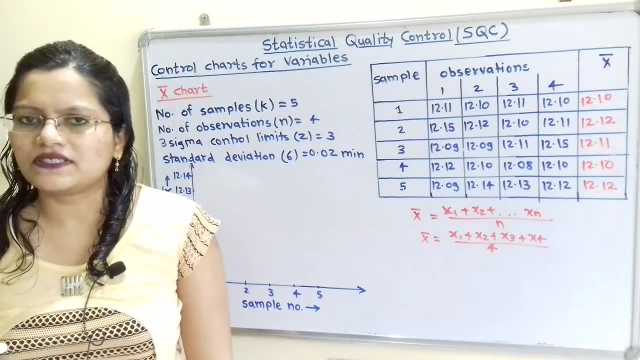 to show the sample number. so there are total five number of samples. so we will start from 0, 1, 2, 3, 4, 5. so at equal distance we have to plot this number. so you can take here one centimeter, two centimeter, as per the space available, and on vertical line we have to plot. 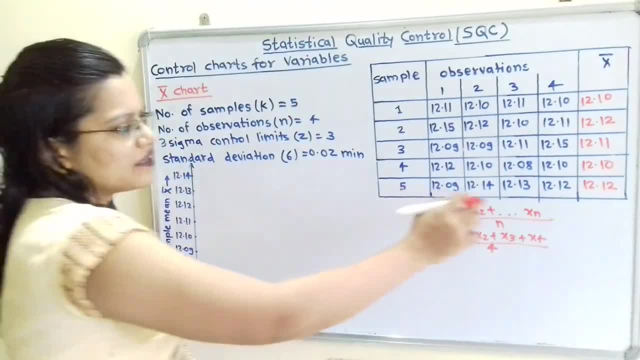 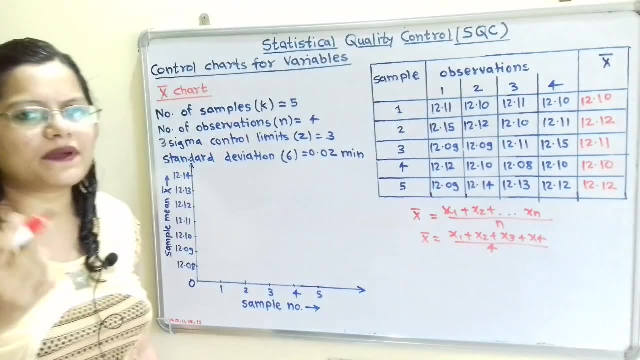 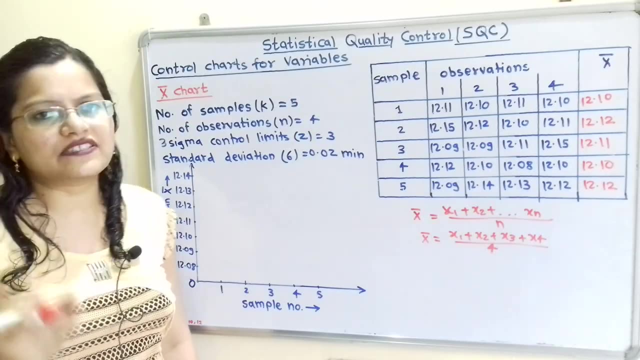 this value of x bar. now, if we observe here, this range is from 12.10, 12.11 and then 12.12. so approximately we have to start from this 12 number, or we can say 12.05 or we can say 12.08. so i have. 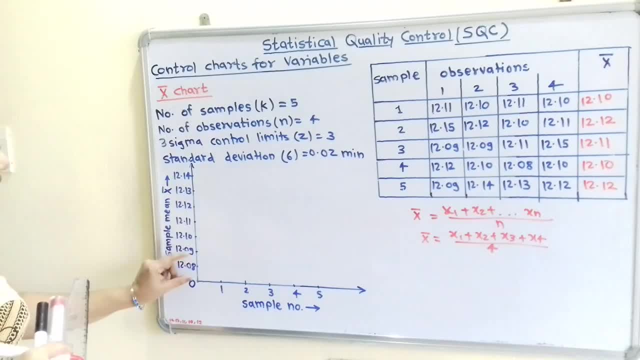 started here from this 12.08, so keep here some sufficient space after zero. and we have to start it from 12.08, 12.09, 12.10, 12.11, 12.12, 12.13 and 12.14. so for these numbers to plot these numbers, 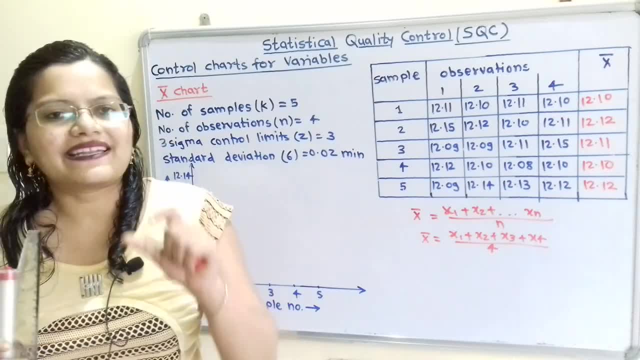 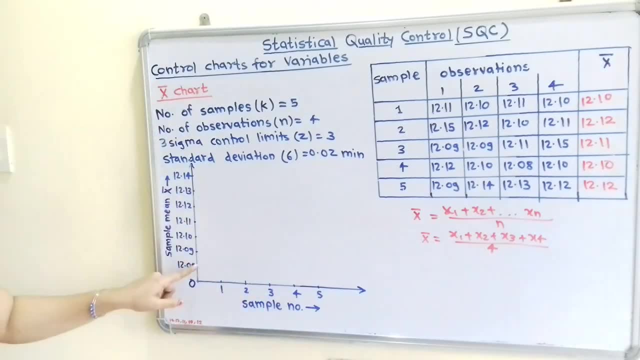 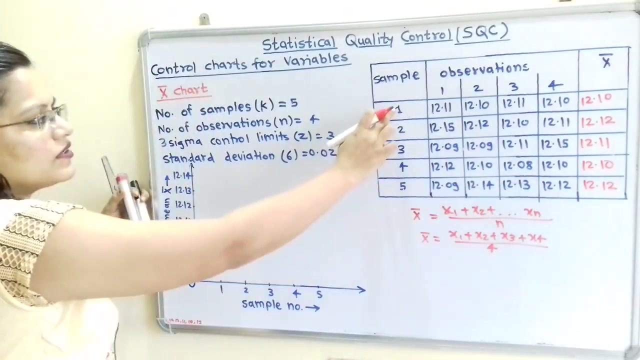 we have to consider some sufficient space. that is, we will take the equal distance, that is, one centimeter. you can also take two centimeter as per the space available. so important question is that we have to keep this equal distance, we have to plot this number at equal distance. apart now how to plot these numbers. so for for the first sample, so if i 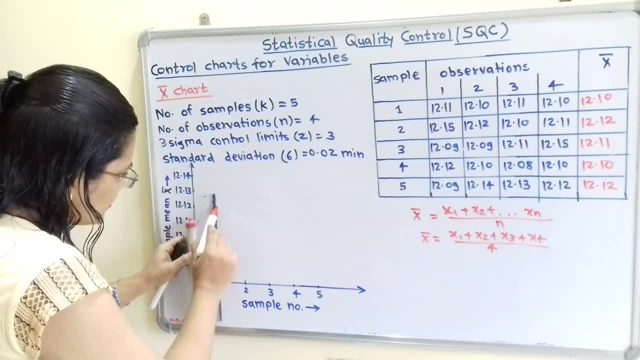 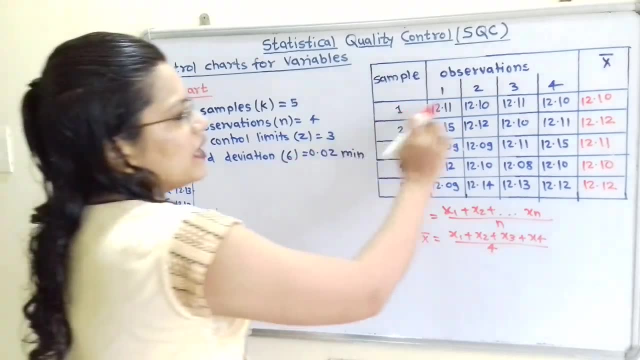 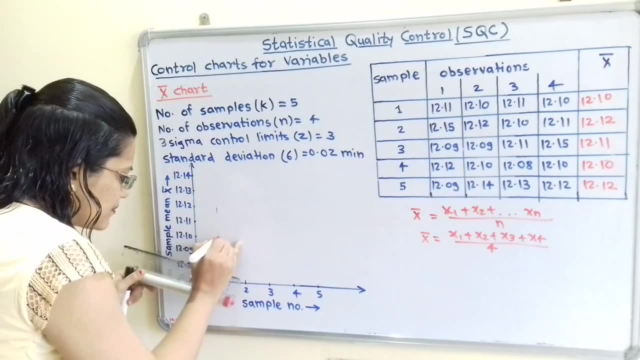 observe. here is the vertical line for the first sample. so this is the rough line i will draw here. and around this vertical line we have to plot 12.10. so 12.10 is here. so i will show here one point with the help of red marker, then the next. 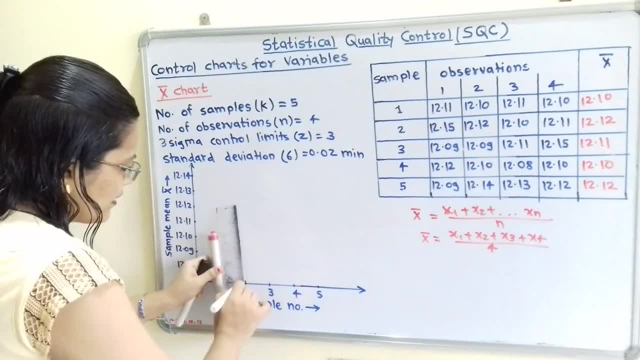 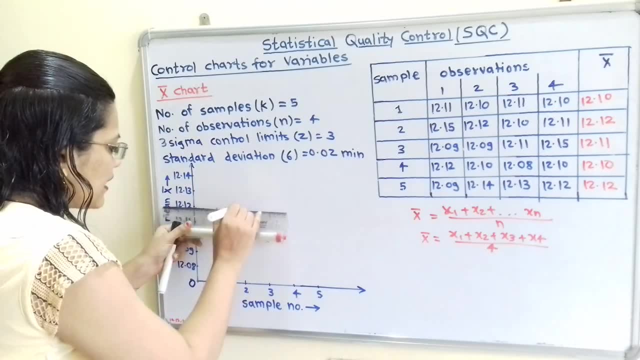 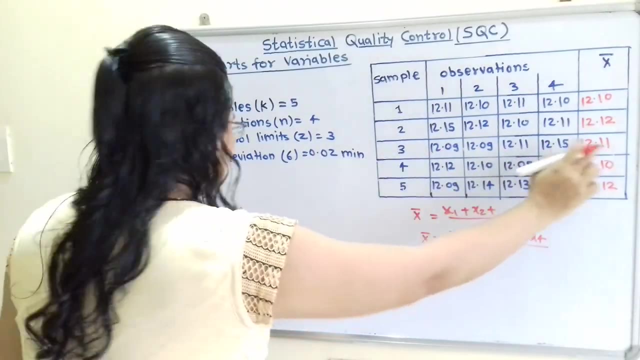 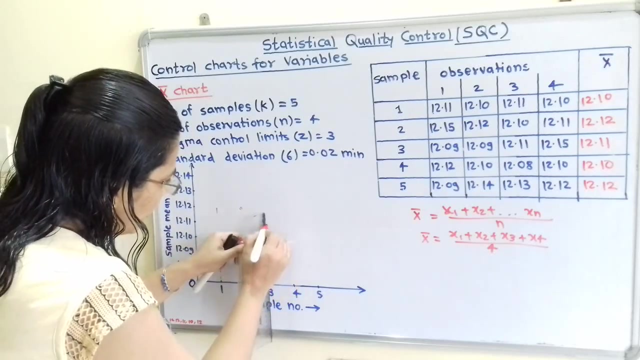 for the second sample it is 12.12. so here is the second sample number. so along this vertical line we have to plot here 12.12. so we will take here the horizontal line and vertical line. so here is this point. then for the third point, this 12.11. so for this 12.11, along this horizontal line and vertical. 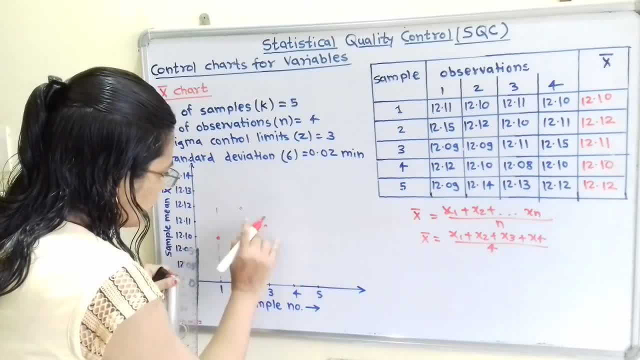 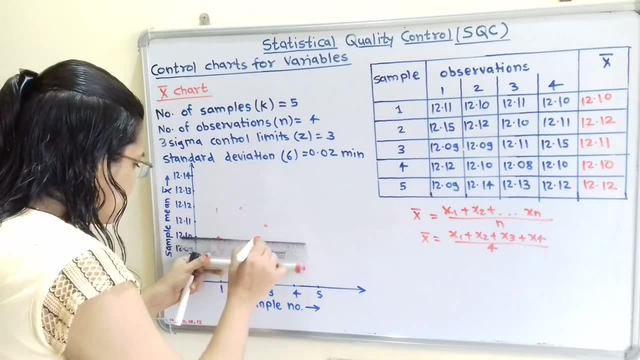 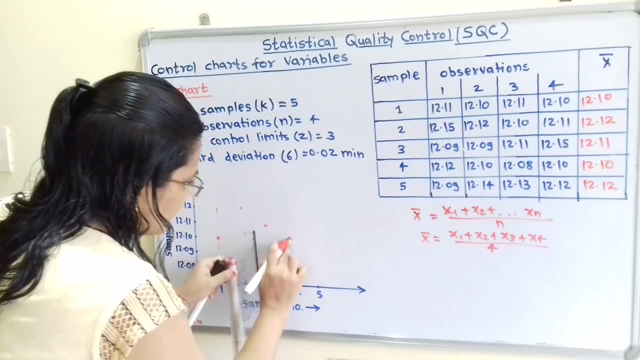 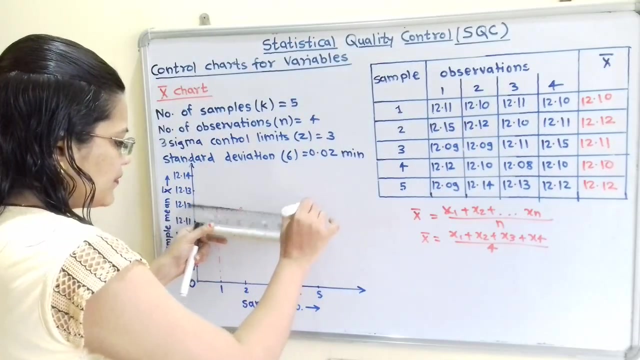 line we have to plot here the third point, that is for 12.11.. Then for the fourth sample: 12.10.. So for the fourth sample again it is 12.10.. Then for the fifth sample it is 12.12.. So here is the fifth sample, Then here is the 12.12.. 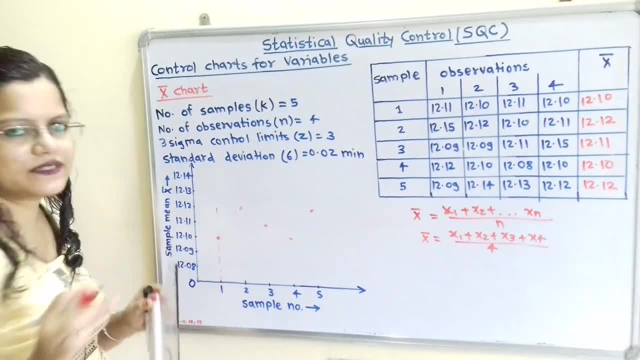 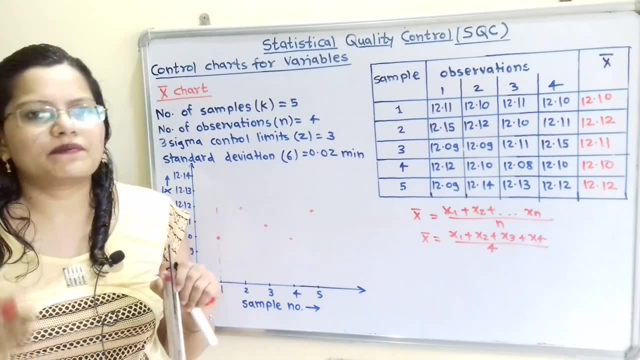 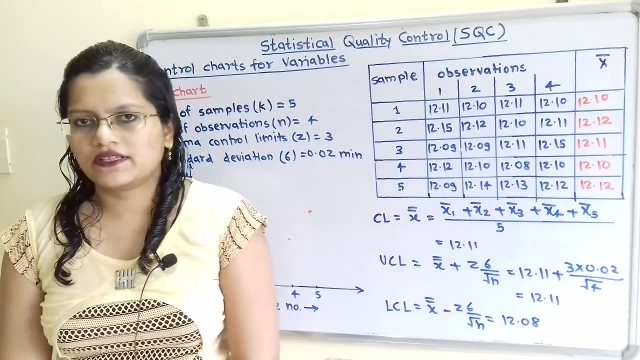 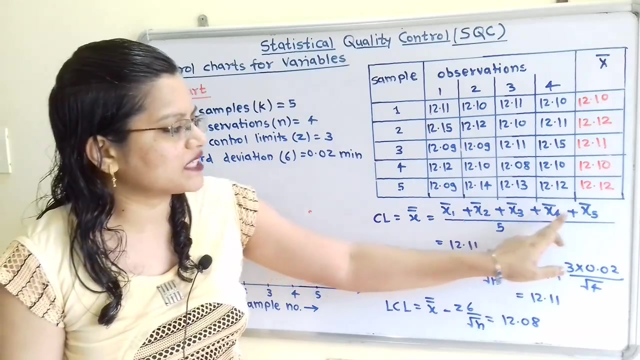 So we have to show these points Now. we will decide centerline upper control limit and lower control limit by using important formulas. We will calculate the value for x double bar, that is, for the centerline CN, and formula is: x1 bar plus x2 bar plus x3 bar plus x4 bar plus x5 bar divided by 5.. 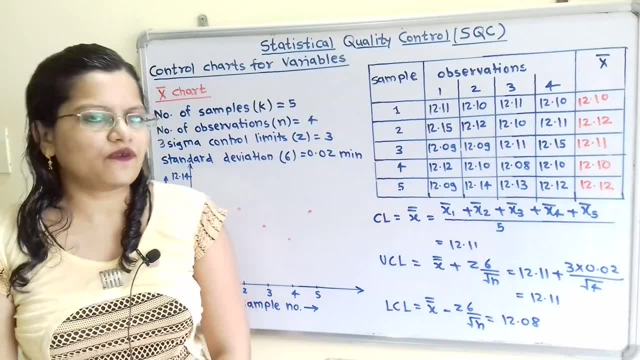 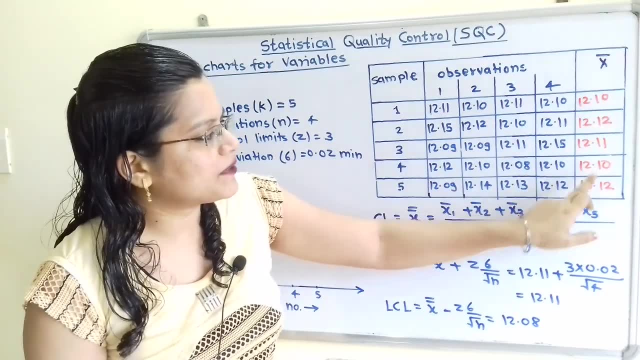 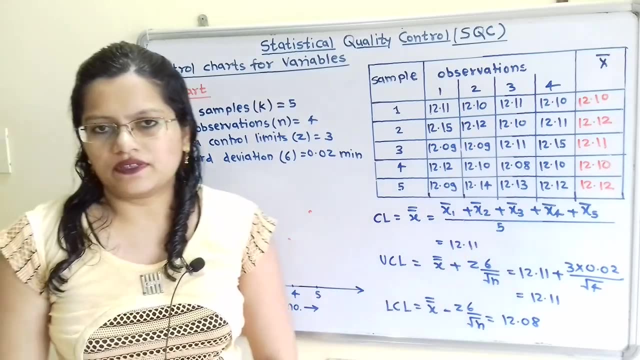 Because there are total number of points, So we have to consider these values, that is, 12.10 plus 12.12 plus 12.11 plus 12.10 plus 12.12 divided by 5, and which is equal to 12.11.. 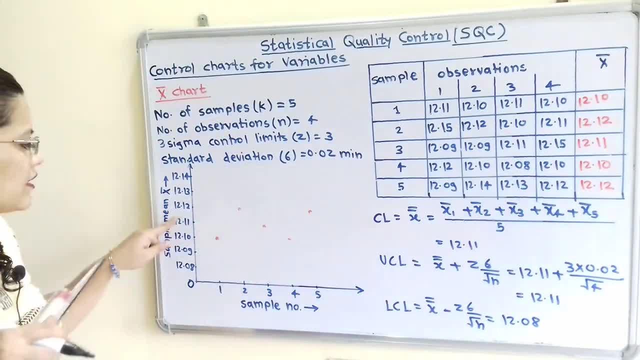 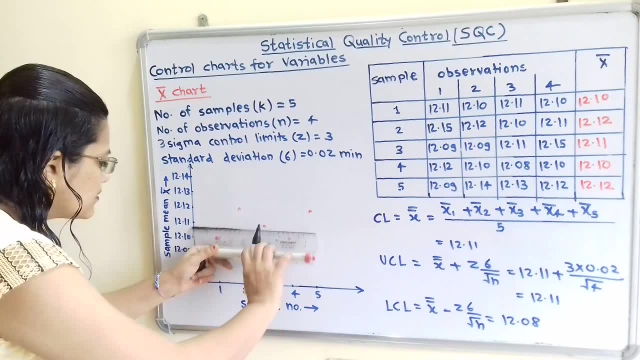 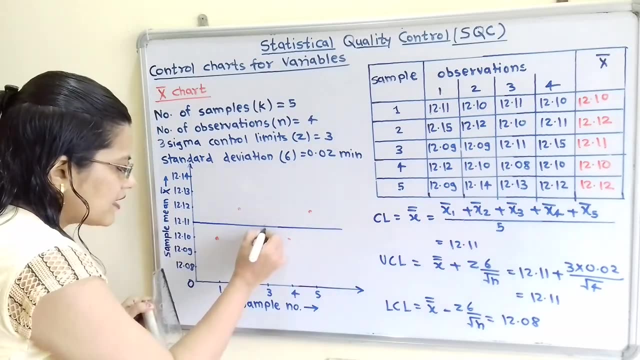 So this is the centerline, So we will draw here one centerline at the point 12.11.. So here is the 12.11.. So we will consider here one horizontal line And this point lies on this 12.11, and this is known as CN. 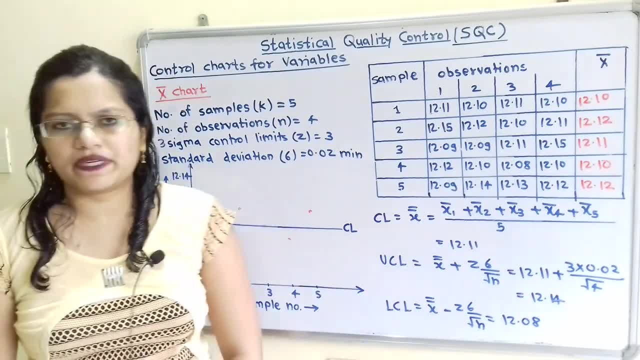 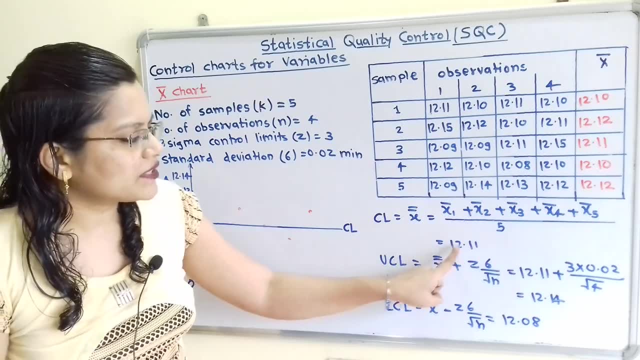 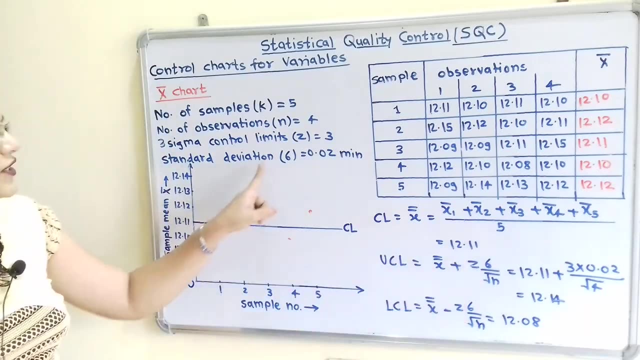 Now we will calculate the next upper control limit, which is equal to x double bar plus z sigma, by under root of n. So here: x double bar, that is 12.11, plus z, value of z is 3 sigma, that is the standard deviation, 0.02 under root of n. 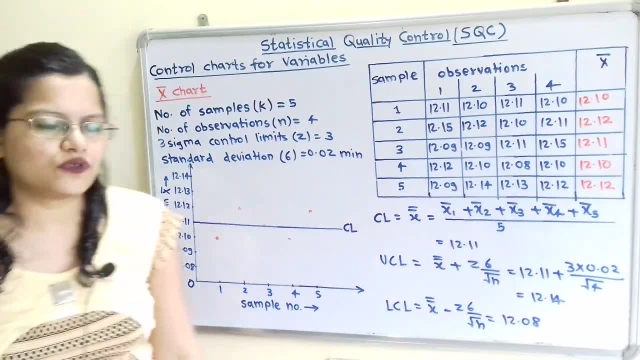 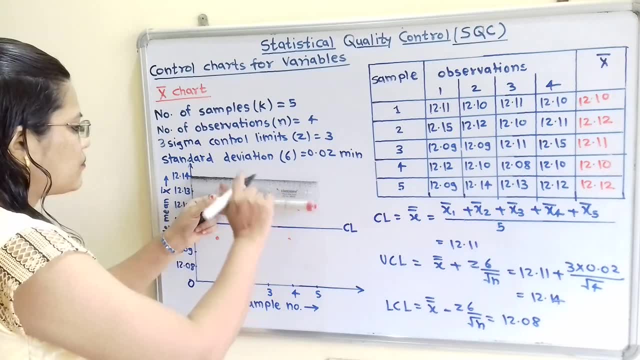 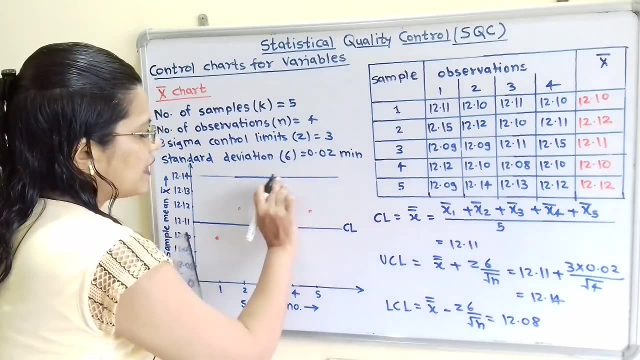 So there are value of n, that is 4.. That is under root of 4.. So when we calculate this we will get 12.14.. So again, I will draw here one horizontal line for 12.14.. And this is the upper control limit. So we have to mention here upper control limit. 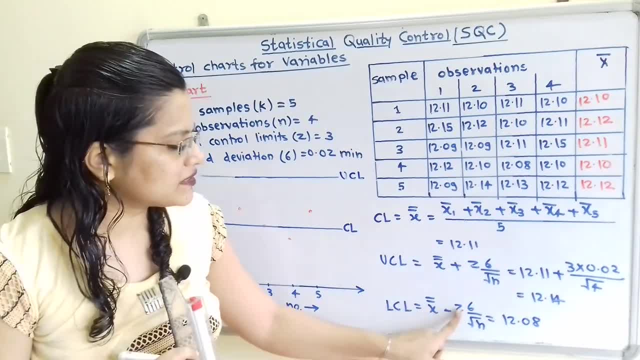 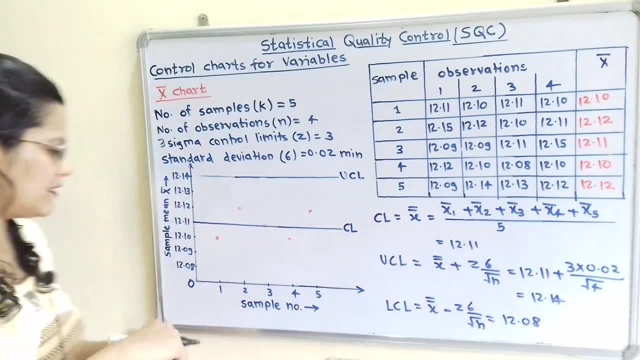 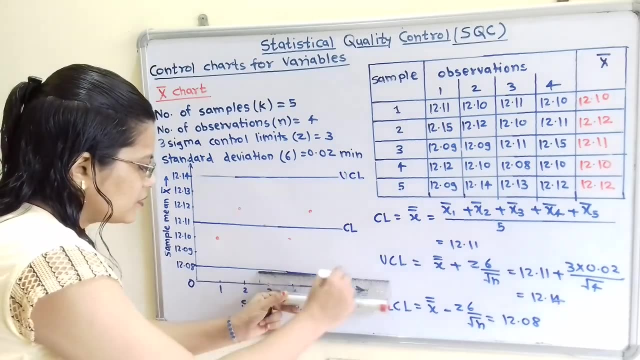 Now for this lower control limit: x double bar minus z sigma by root n. So if we calculate by putting the value, then it is 12.08.. So I will draw here one horizontal line for 12.08.. So this is the lower control limit. So we have to mention all these. 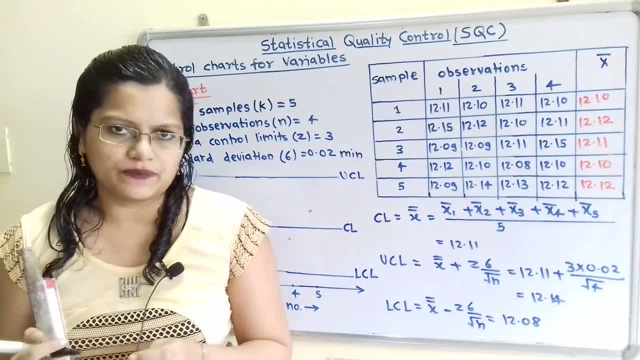 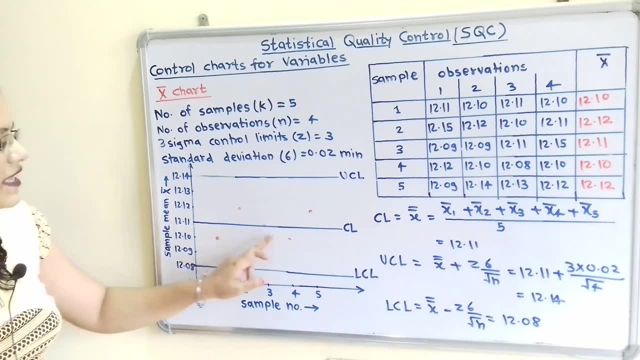 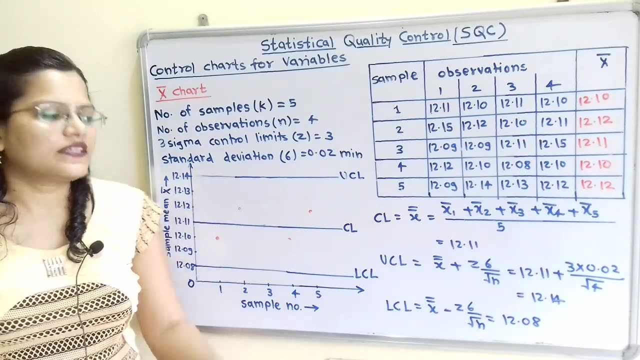 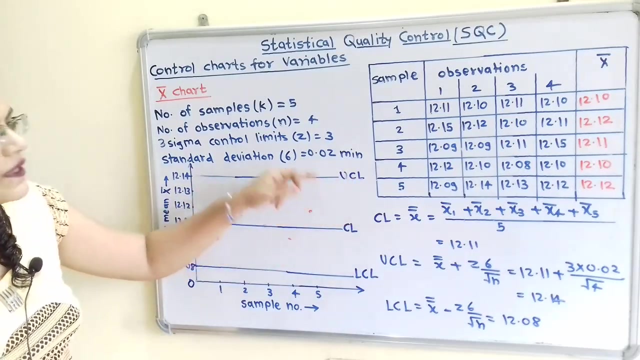 Now we have to write the answer by observation. Now, if we observe here all these readings, that is, all the points, lies under this lower control limit and upper control limit, That means we can say that this process is Is under control. So no, any point cross the boundary for this upper control limit and lower control limit. 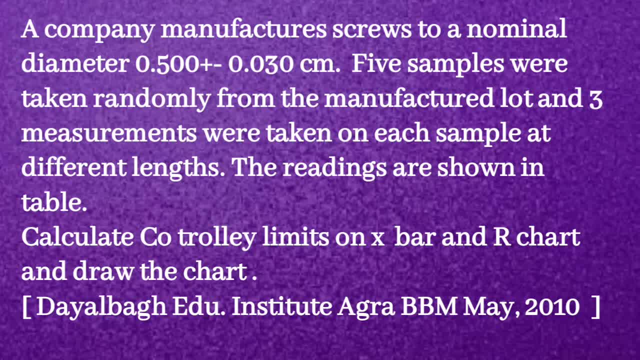 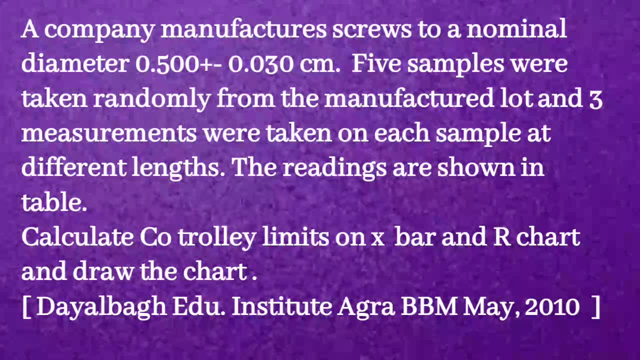 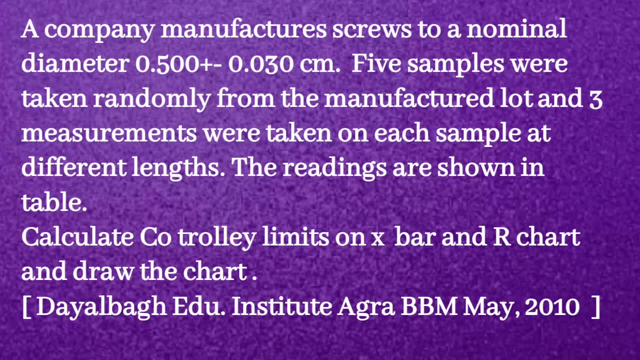 Given question. A company manufactures screws to a nominal diameter 0.500 plus minus 0.030 centimeter. Five samples were taken randomly from the manufactured lot and three measurements were taken On each sample at different lengths. The readings are shown in the table. 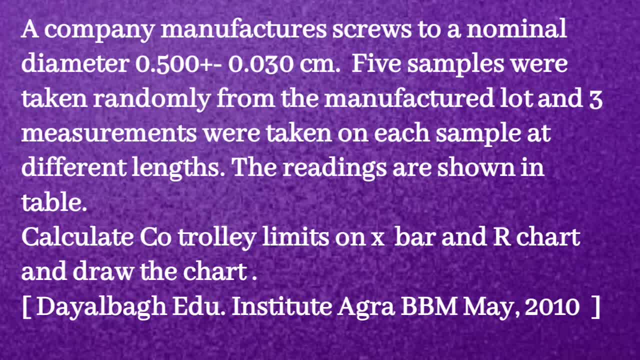 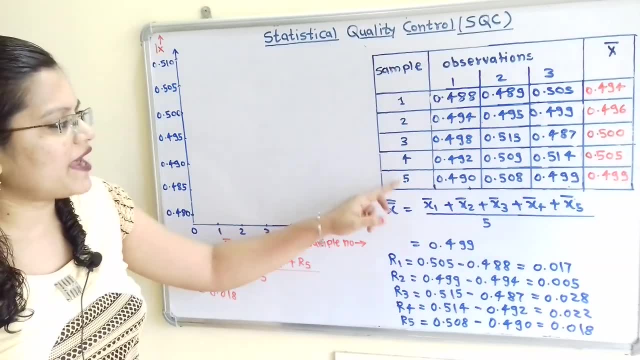 Calculate the control limits on x, bar and R charts and draw the charts? This question was asked Dyalbagh Education Institute, Agra, BBM, May 2010.. This is the given table. There are five number of samples and for each sample there are three observations. 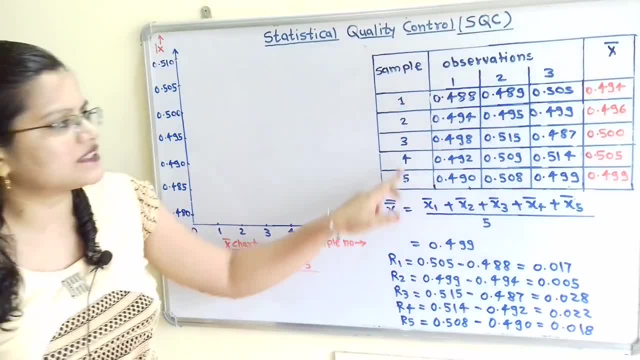 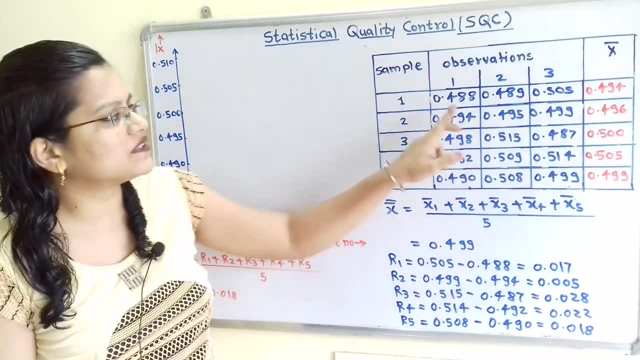 So first, First step is to calculate X bar for each sample. So how to calculate this? So we have to add all these numbers for the three observations, that is 0.488 plus 0.489 plus 0.505 divided. 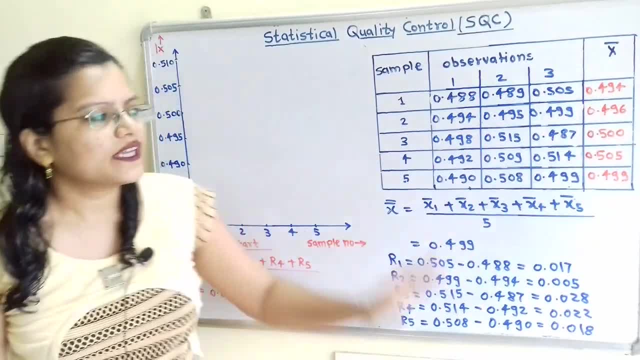 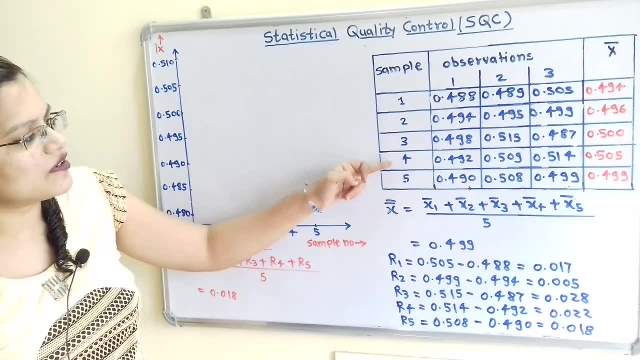 by 3.. Answer is 0.494.. In the same way, we have to calculate the value of X bar for these other samples, that is, 2nd, 3rd, 4th and 5th. and here are the values. Now we will calculate. 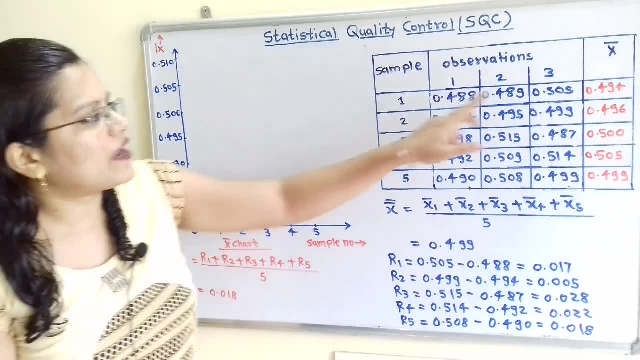 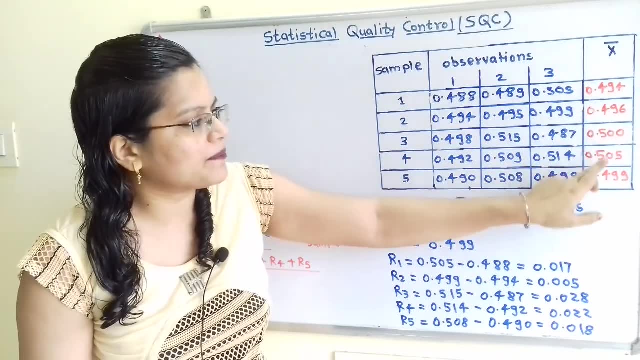 X double bar. So how to calculate this? So value of X bar. for the first sample, we will consider this as X1 bar. this is X2 bar, X3 bar, X4 bar and X5 bar. So X double bar is: 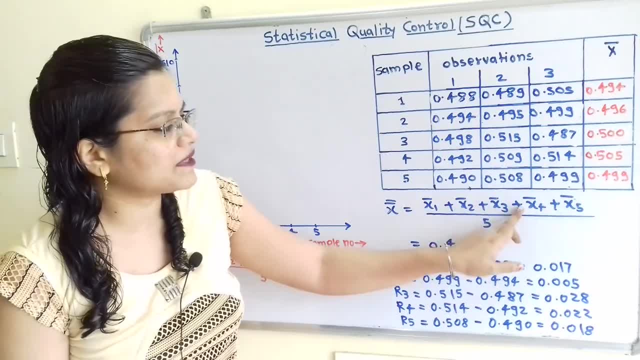 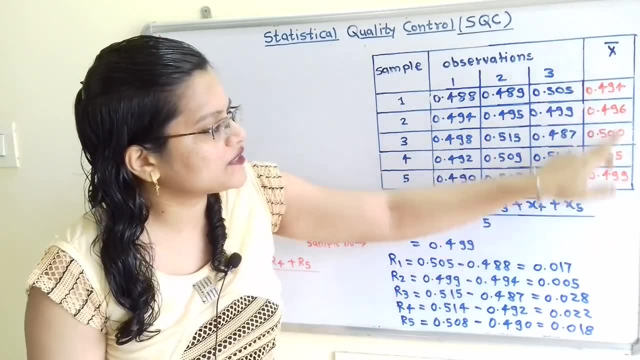 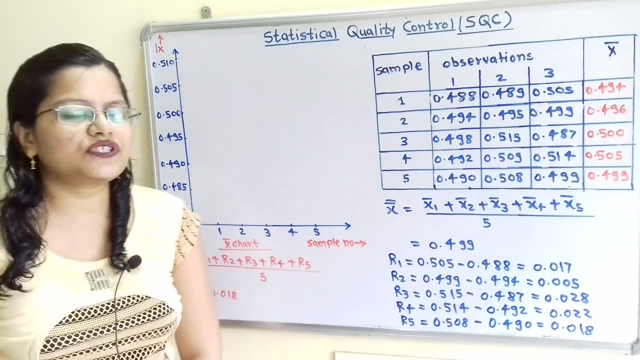 equal to X1 bar plus X2 bar, plus X3 bar plus X4 bar plus X5 bar, divided by 5.. So when we calculate this, when we add all these values and divide it by 5, then the answer is 0.499.. Now in this question we have to calculate the value of R also. So how to calculate this range R, That is, for each number of sample, we have to select the maximum value of X and minimum value of X. So for sample 1,, maximum value of X is 0.494.. That is, the maximum value of this observation is 0.505 and minimum value is 0.488.. So when 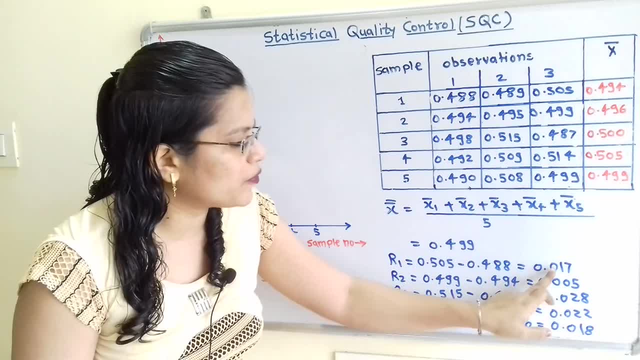 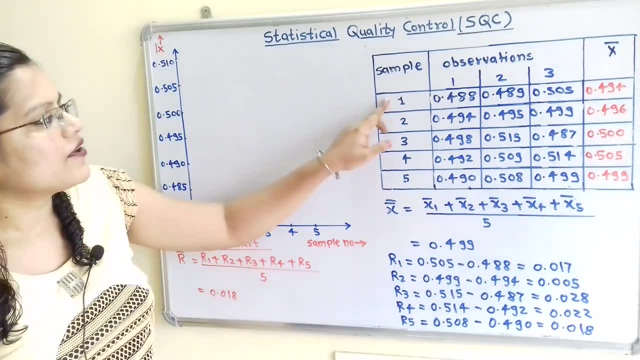 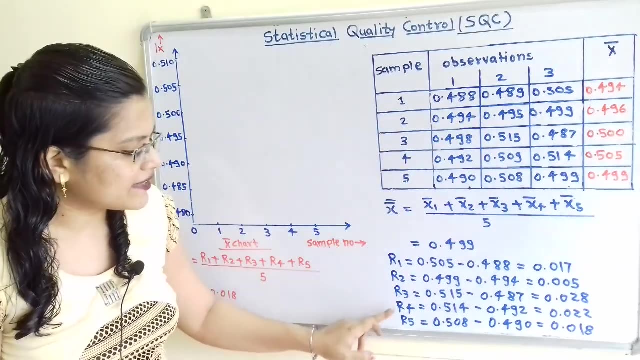 we take the difference, then we will get the answer 0.070.. Now, in the same way, we have to calculate the other values, That is, range for sample 1 is known as R1,, range for sample 2 is known as R2, R3, R4 and R5.. So here are the values. 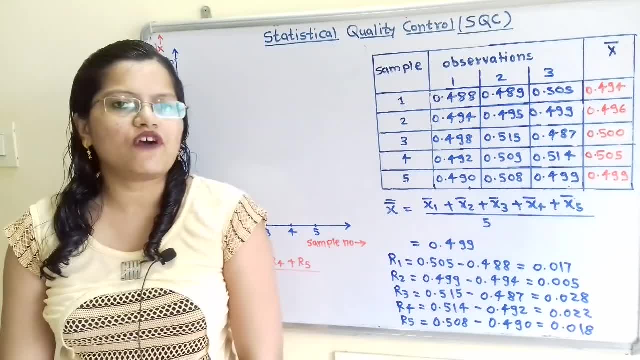 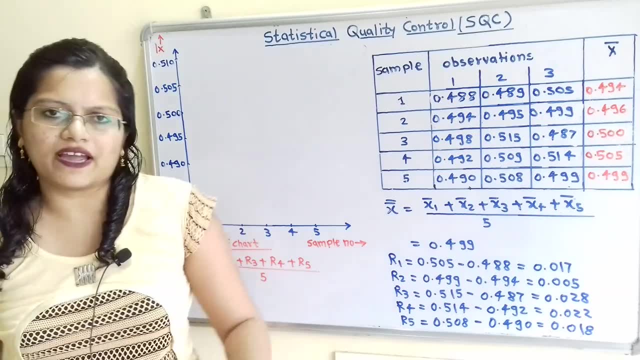 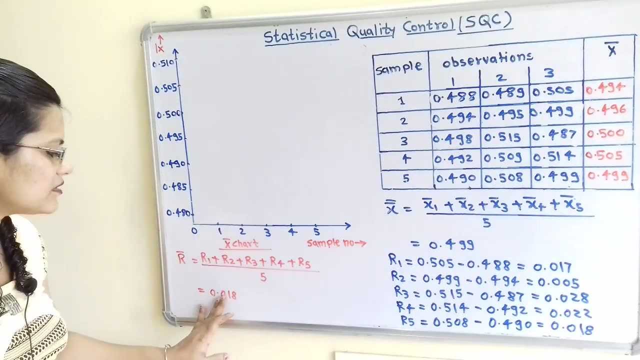 Now from these values we can calculate the value of R bar. That is equal to R1 plus R2 plus R3 plus R4 plus R5 divided by 5.. So when we add all these values and divide it by 5, then the answer is 0.018.. Now how to plot the X bar chart. So on horizontal line, 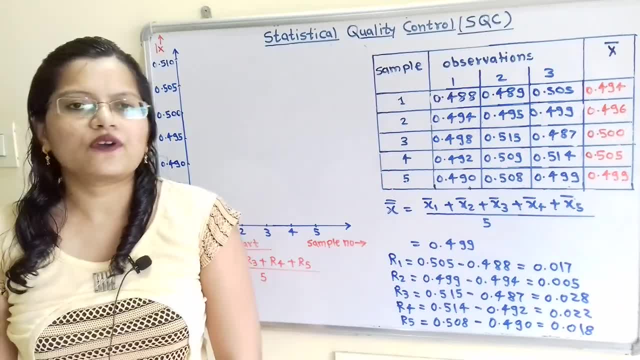 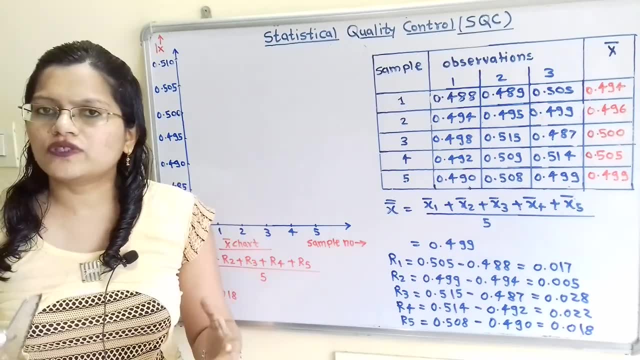 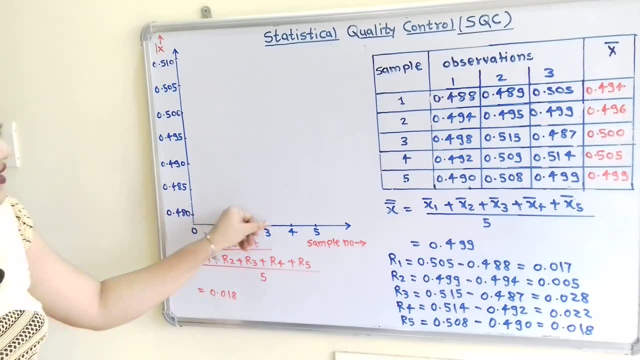 we have to plot the number of sample. There are total 5 numbers, So we have to take the equal distance. So you can take 1 centimeter, 2 centimeter, as per the space available, and we will plot here. So we will start from 0,, 1,, 2,, 3,, 4,, 5.. On. 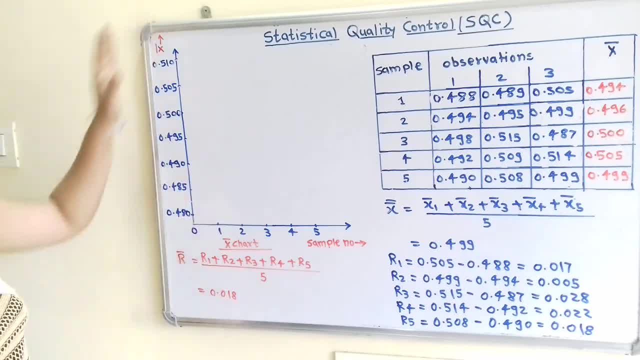 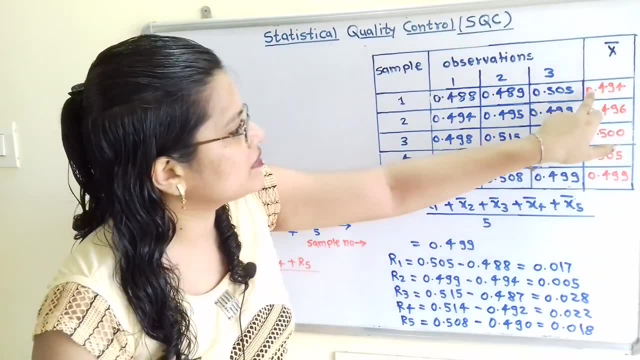 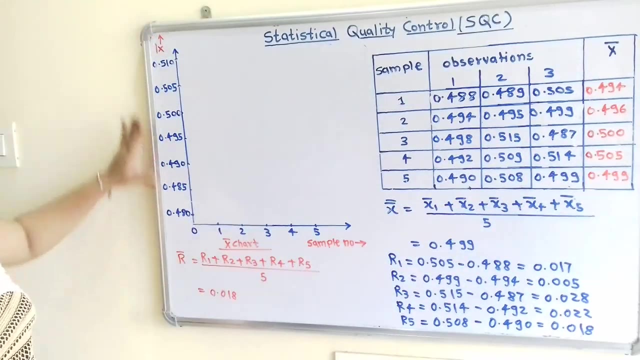 this horizontal line there is sample number and on vertical line we have to plot the values of X bar. Now if we observe here, minimum value is 0.494 and maximum value 0.505.. So nearby this, we have to start from the plotting the value. So I will start from. 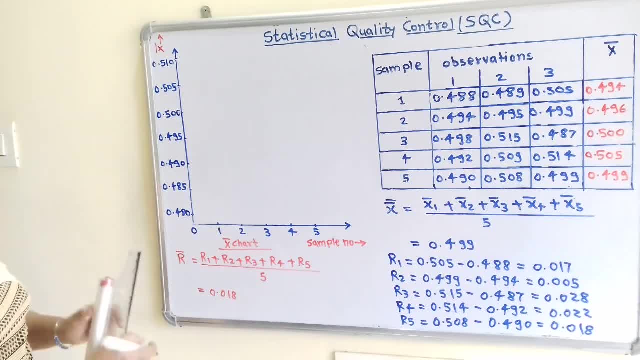 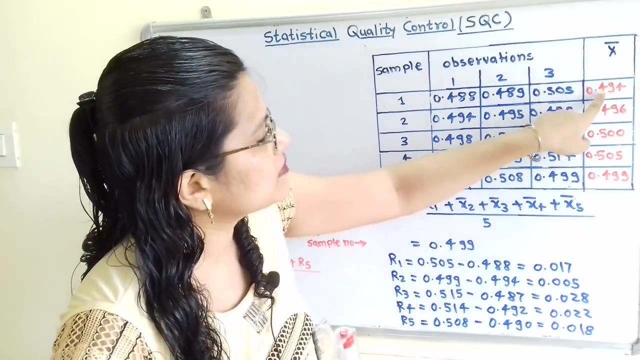 0.480.. So if I take that is the first value as 0.480, then in between this 0.480 and 0.490, I will take this 10 centimeter, because these are the values, that is, 494, 496.. So for the 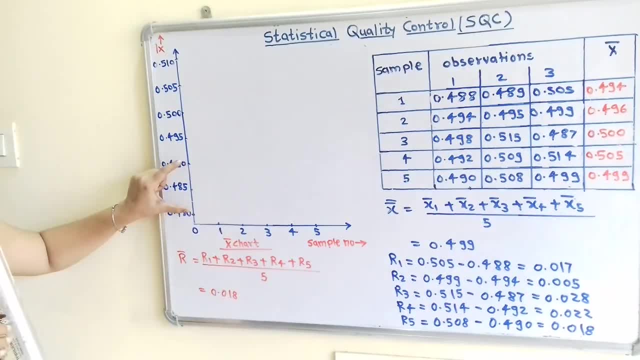 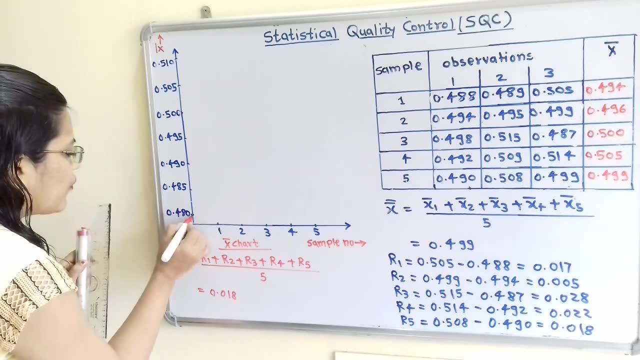 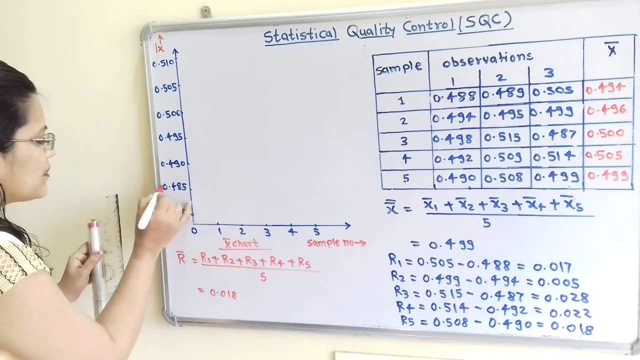 standing purpose. I have taken here the 10 centimeter distance. You can take 5 centimeter if space is not available. So here in between, 0.480, I will take here 0.490.. But in between that middle point, that is, after 5 centimeter, I will take here 0.485.. So again here after. 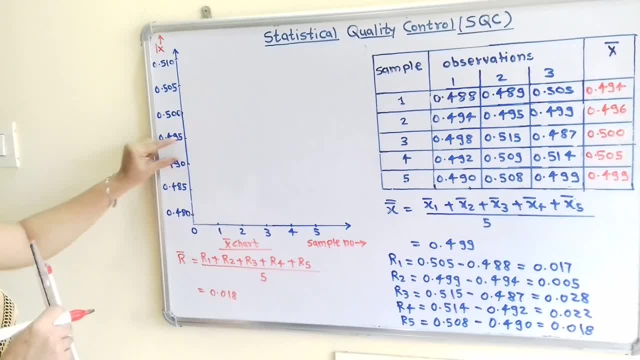 0.490, after 5 centimeter I will take here, or I will show here one point for 0.485.. So I will take here 0.495, then 0.500, 0.505 and then 0.510.. So these are the points. 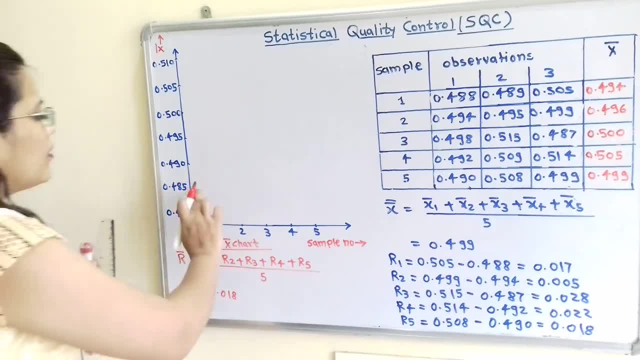 that we have to plot Now how to make here the points. So for the sample number 1, so here is the vertical line for sample number 1.. Value is 0.494.. So here is 490 and here 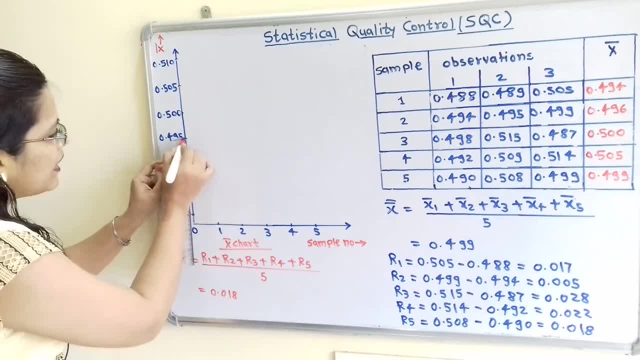 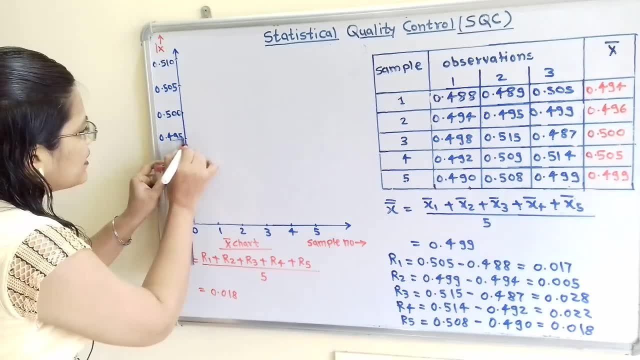 is 495.. So here distance in between is 0.495.. So here is 0.495.. So here is 0.495.. So in between them, that is, in between 490 and 495, is 5 centimeter. So if I take 1 centimeter, 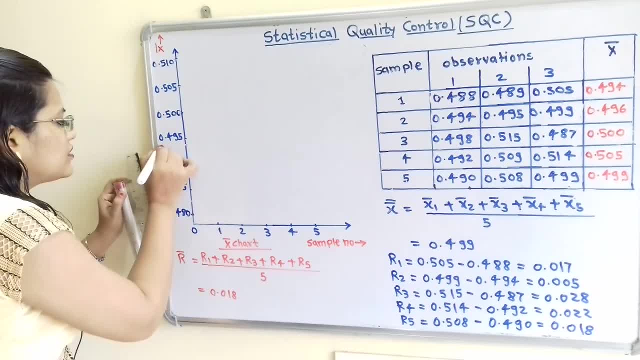 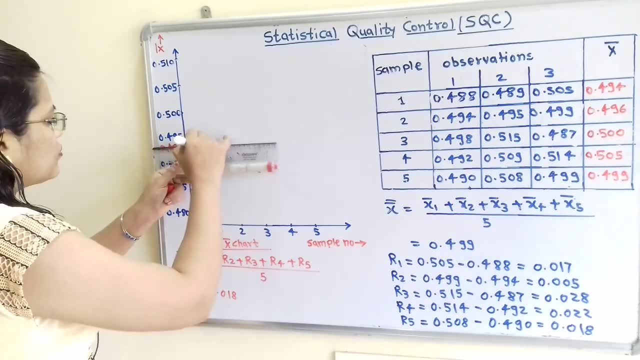 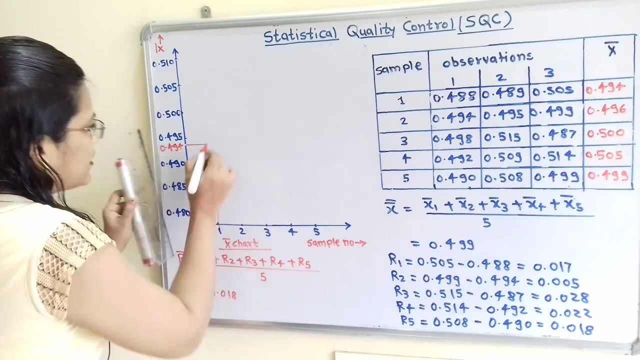 earlier than this 495, then here is 0.494.. So I will take here the point of intersection. So if I draw here rough line that is from 0 and this is the vertical line, then here is the point of intersection. So this point of intersection is our 495.. So here is the 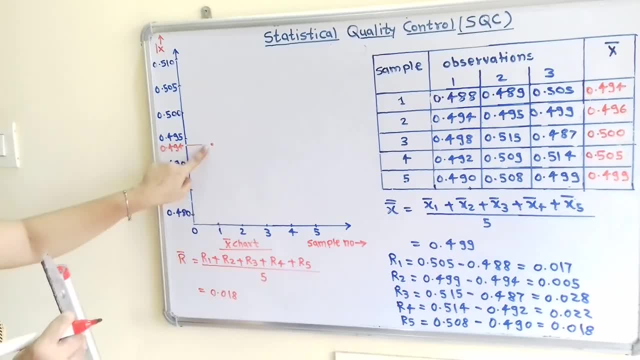 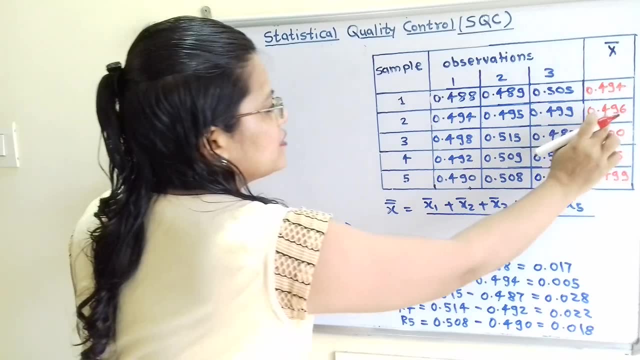 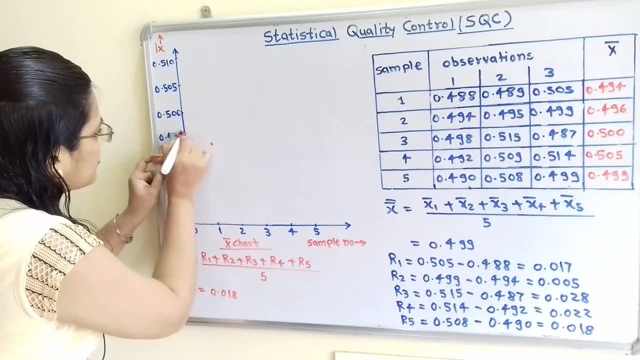 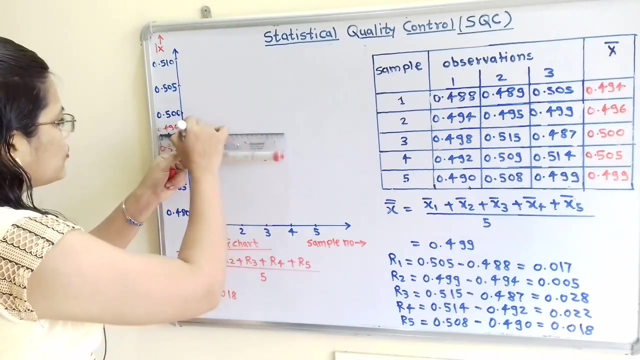 first observation. So I will remove these rough lines, Then we will move next. that is for second sample. it is 0.496.. So here is 0.495.. So after that 1 centimeter, here is 0.496.. So again, I will take here one horizontal, rough horizontal line and from sample number: 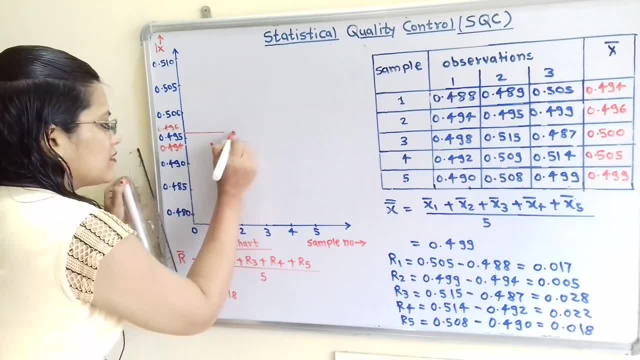 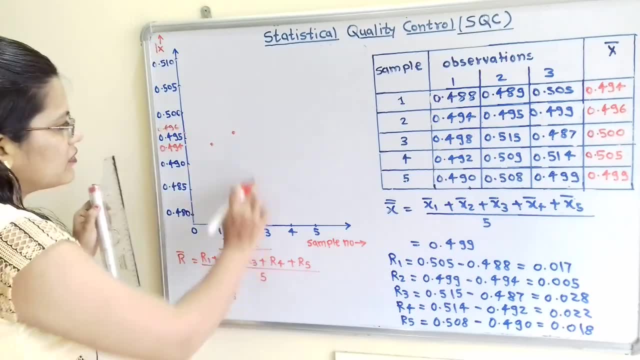 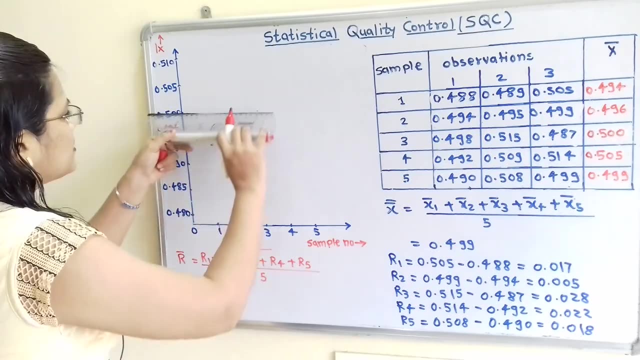 2, here is the vertical line. So here is the horizontal line. and from sample number 2, here is the horizontal line. So this is our second reading, Then 0.500. So this is for the third, So here is 0.500.. So if I take here the vertical line, and here is the, 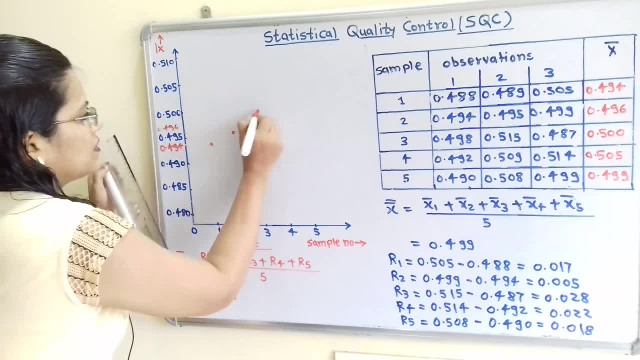 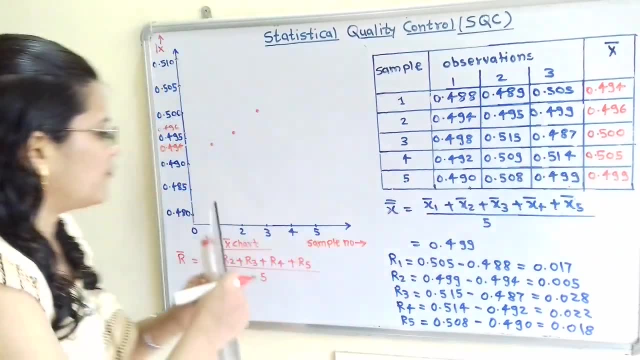 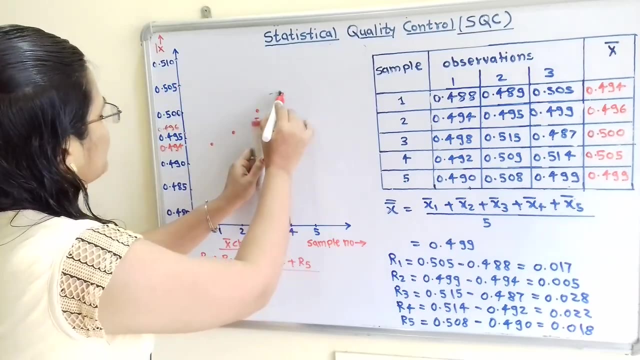 horizontal line, then this is the point of intersection. So this is the reading. for the third sample, That is 0.500.. Then next one, 0.505.. So for the fourth sample, it is 0.505.. So that is also available. So, on this vertical line, and here is the horizontal, 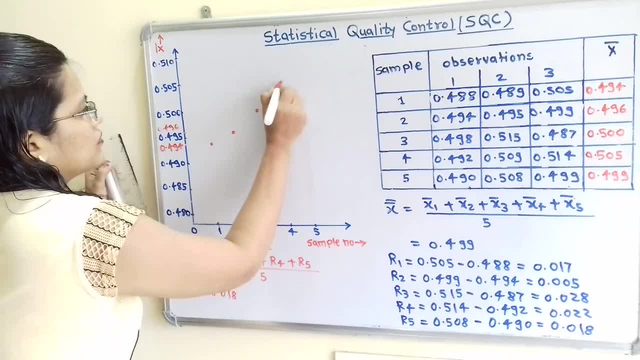 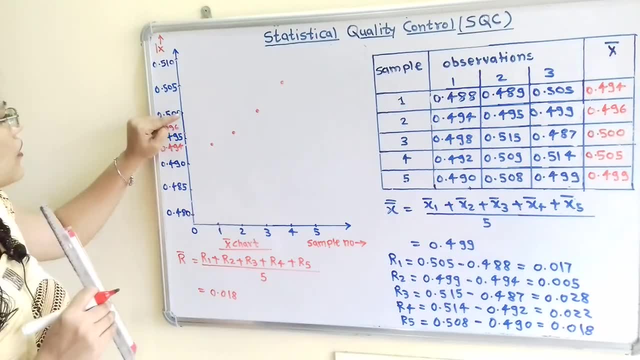 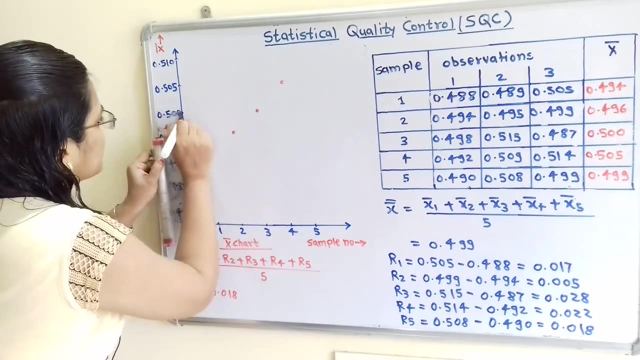 line. So here is the point of intersection, So I will show here this point. Then 0.499.. So if we observe before this 0.500, once if I take one centimeter distance, then here is the value of 0.499.. So this is for the fifth sample. 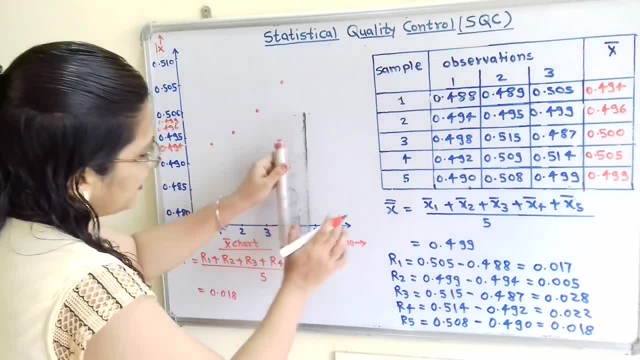 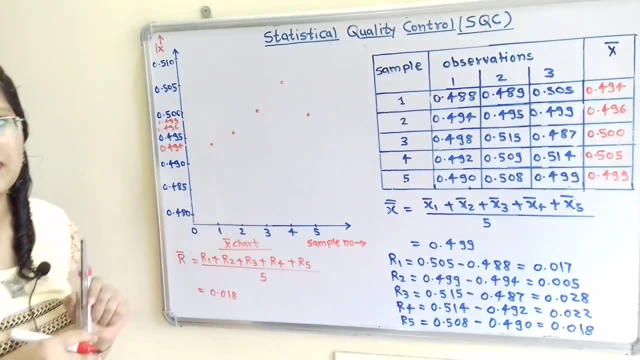 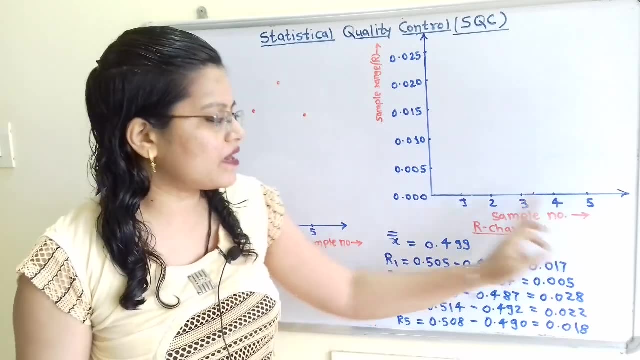 So if I draw here one horizontal line and here is vertical line, then here is the point of intersection. So this is our fifth reading. Now we will prepare our chart On horizontal line. we have to plot the sample number, That is, 1,, 2,, 3,, 4,, 5.. So we have to plot these. 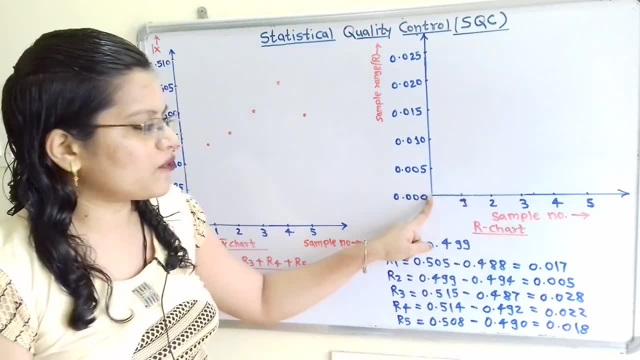 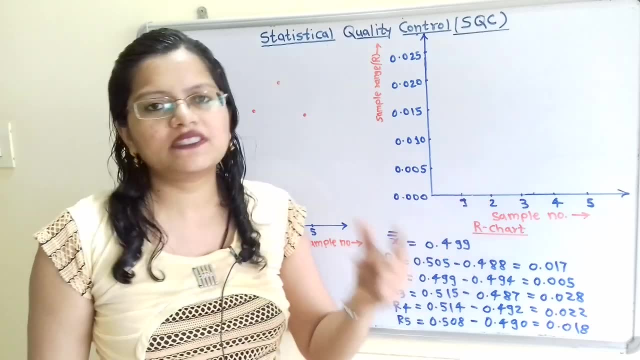 numbers at equal distance apart. So we have to start from 0.. So 0 to 1, suppose there is a distance. then in between 1 to 2, there is same distance, that is 2 centimeter Now. 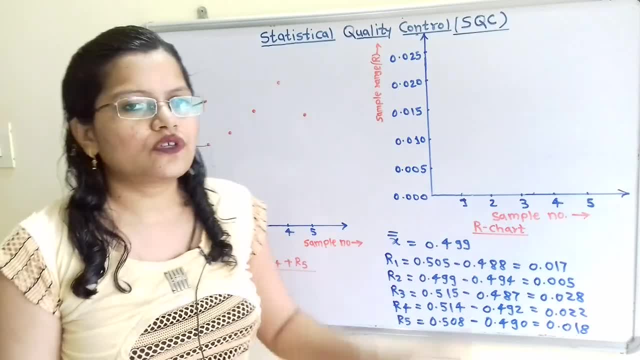 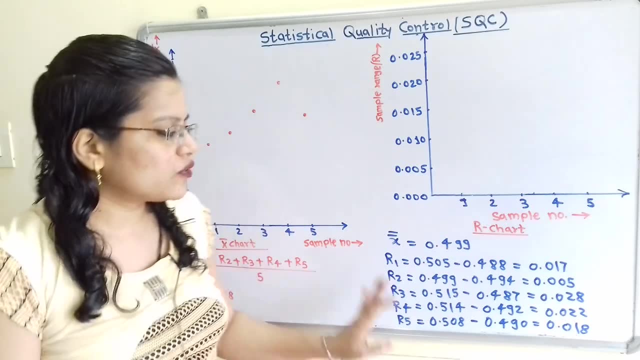 how to plot the numbers on vertical line. So for that we have to refer the values of R1, R2, R3, R4 and R5.. So if we observe here minimum value, 0.005 and maximum value, 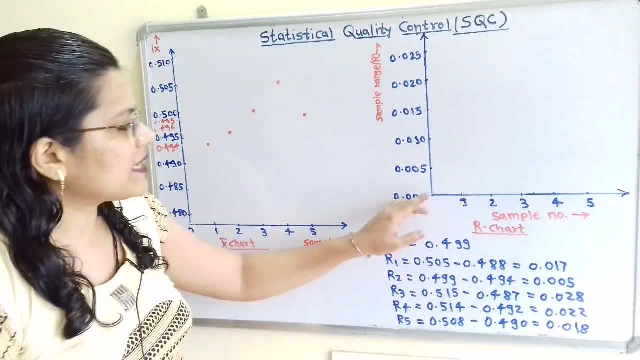 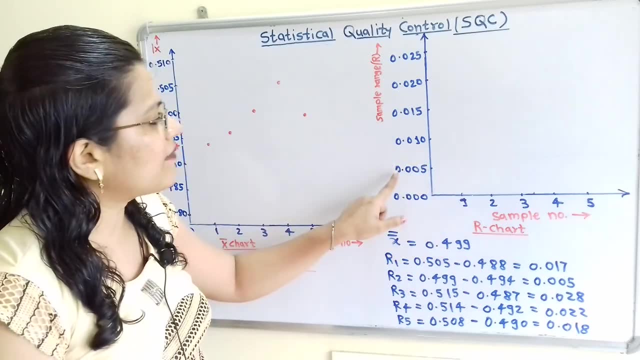 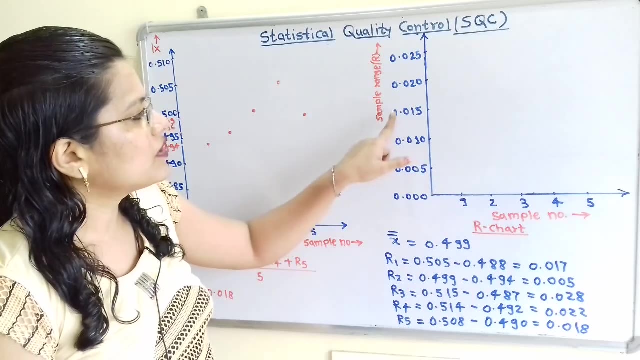 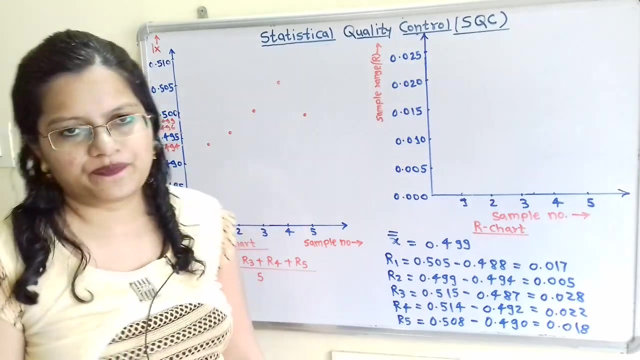 0.028.. So I will take here, or I will start here from this 0.. Then there is 5 centimeter distance and I will take 0.005.. Again, there is 5 centimeter distance, then 0.010, then 0.015, 0.020,, then 0.025.. So in this way we have to plot the. 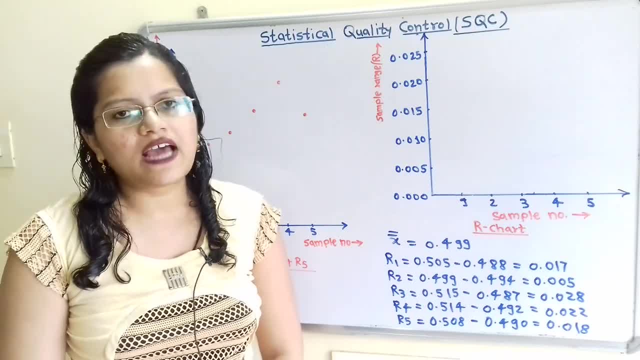 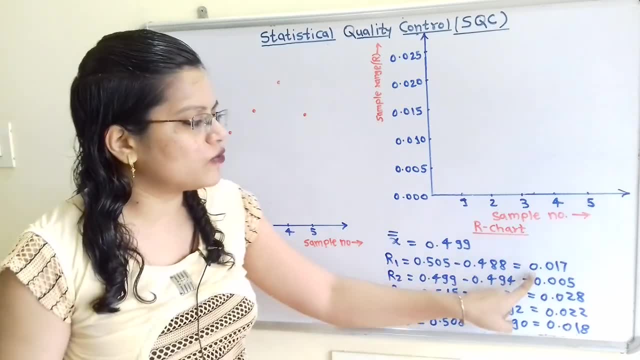 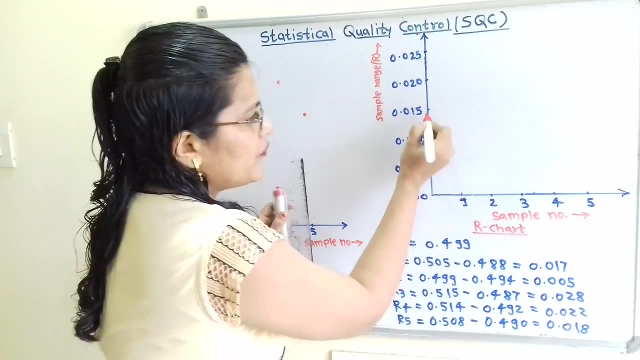 values on the vertical line. Now we will start to plot the values. So first one for R1, that is for sample number 1.. So the value is 0.017.. So for that I will take here after 0.015, there is 2 centimeter. 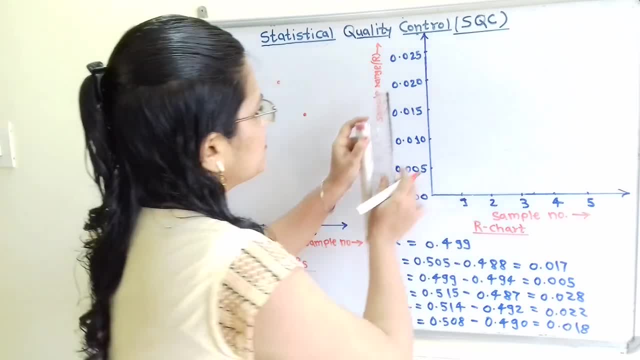 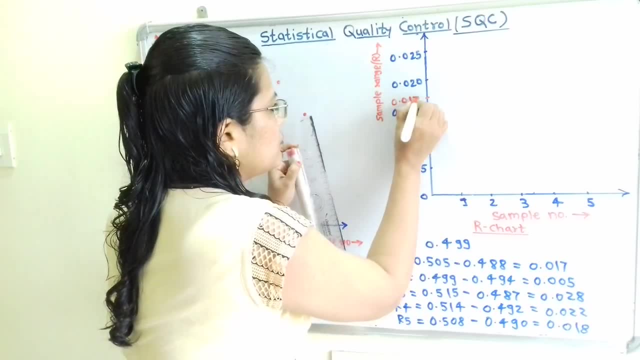 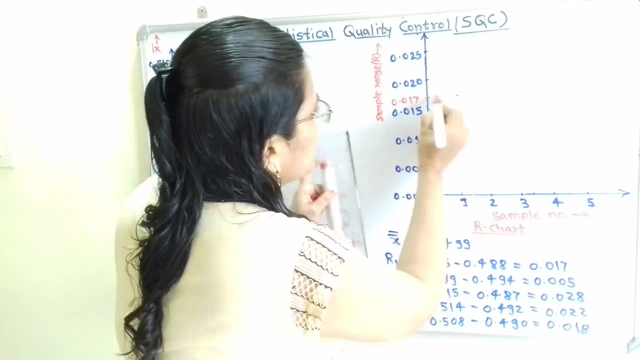 distance, and then this value will be 0.017.. So I will take here the 2 centimeter distance, I will plot here 0.017, and for the sample number 1, I will take here this vertical line, and here is the point of intersection. So this is our first reading. 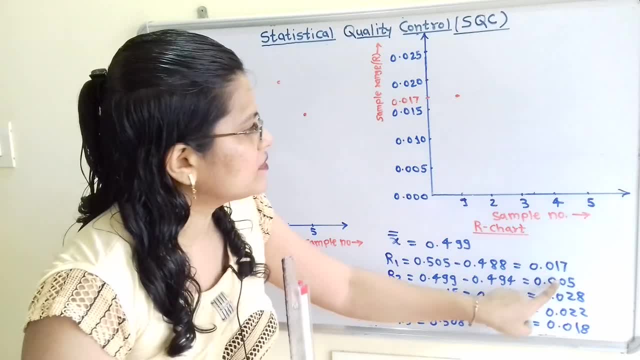 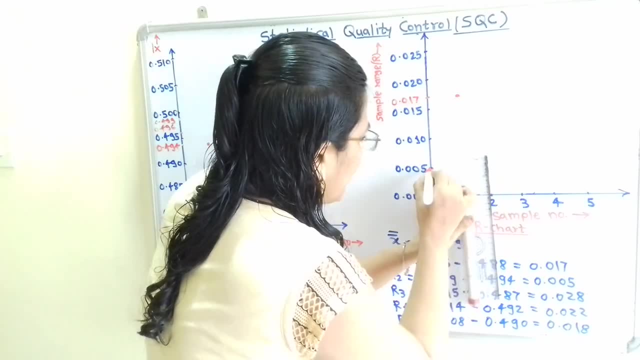 Then the second point: R2, it is 0.005.. So here is 0.005.. So if I take here this vertical line and this horizontal line- here is the point of intersection- Then for R3, it is: 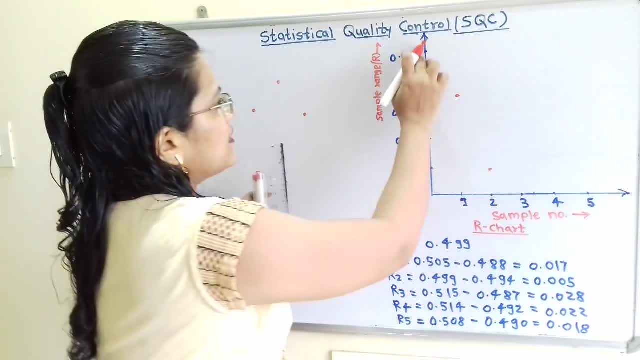 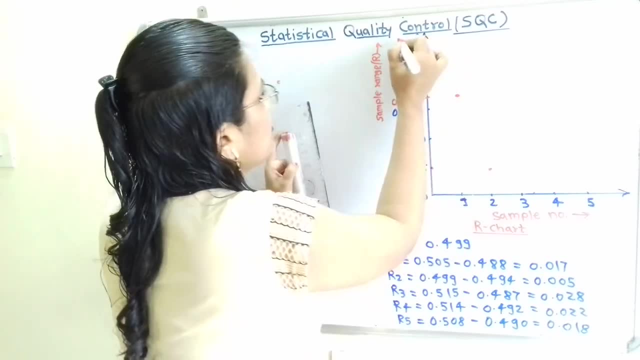 0.028.. So it is 3 centimeter after 0.025.. So I will take here 3 centimeter distance. So point is here. So I will take 0.028.. So I will take 0.028.. So I will take 0.028.. 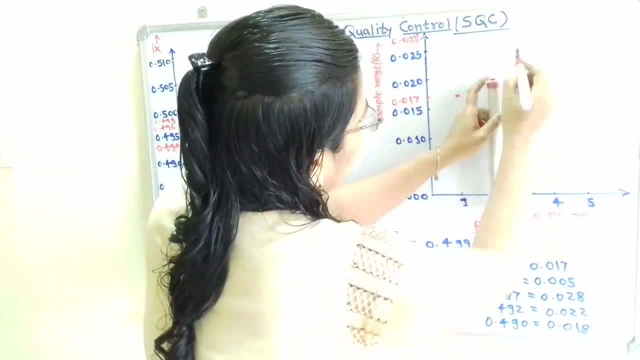 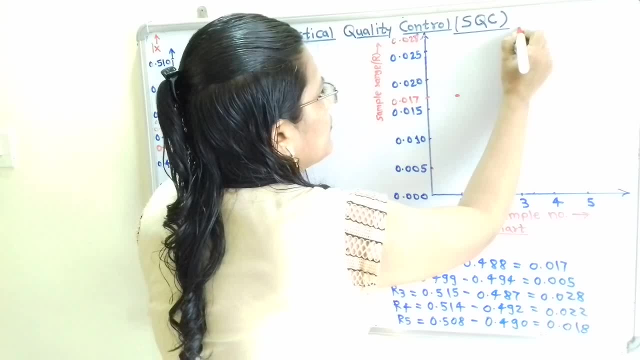 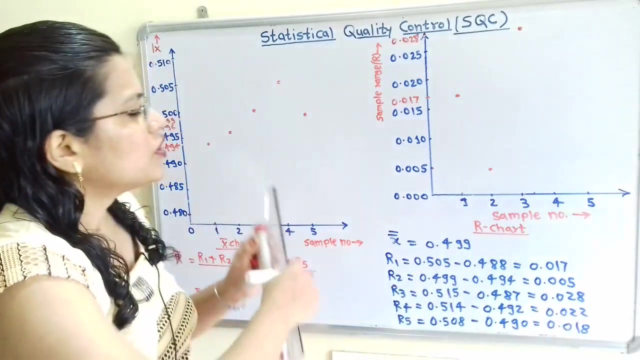 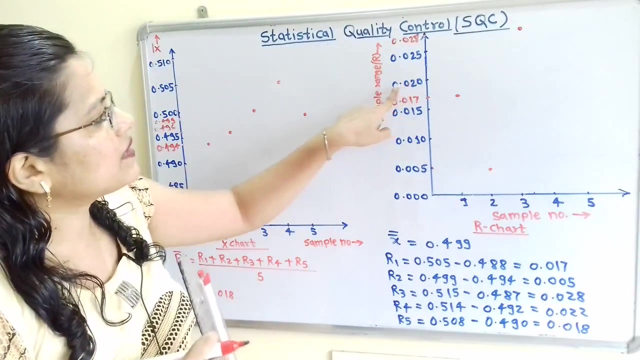 And here is the third sample. So I will take here the vertical line and here is the horizontal line. So this is the point of intersection. So this is our third reading, Then next one: 0.022.. So it is 2 centimeter after 0.020.. Now if we observe, we can say 0.020.. Then 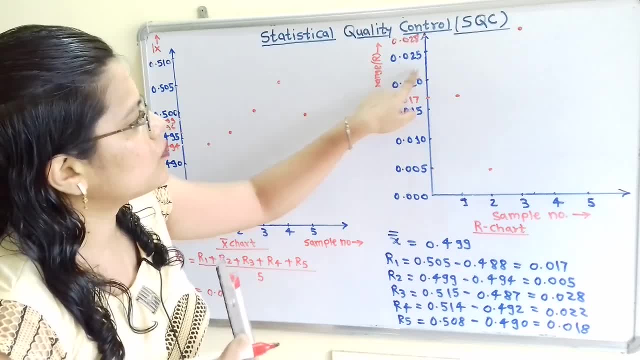 after 1 centimeter 0.021.. Then after 1 centimeter 0.022, 0.023,, 0.024 and 0.025.. So in between 20 and 25, 5 centimeter. 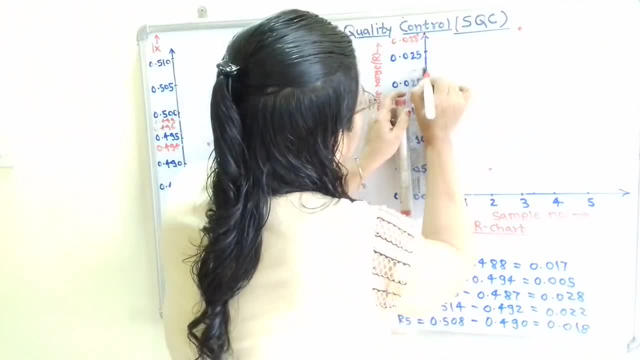 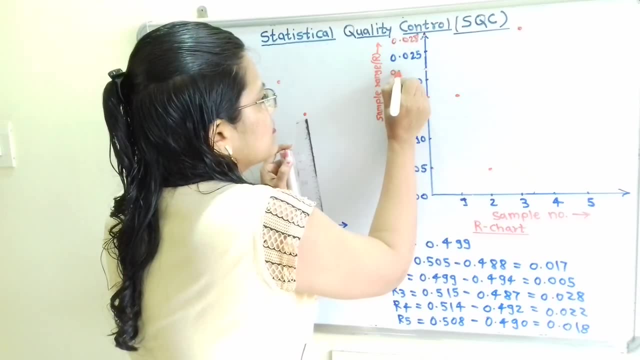 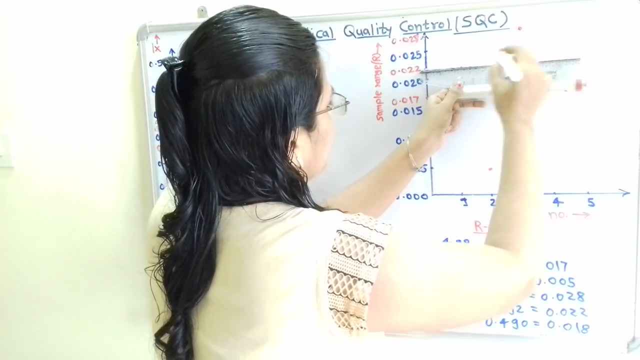 distance. So I will take here 2 centimeter distance and I will mark here 0.022.. Then this is our sample number 4.. So if I take this horizontal line and here is the vertical line, Then here is the vertical line. 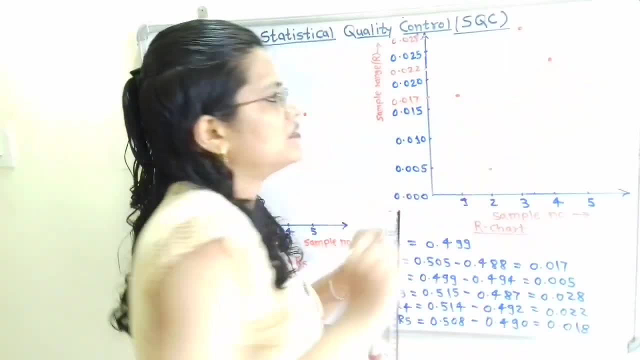 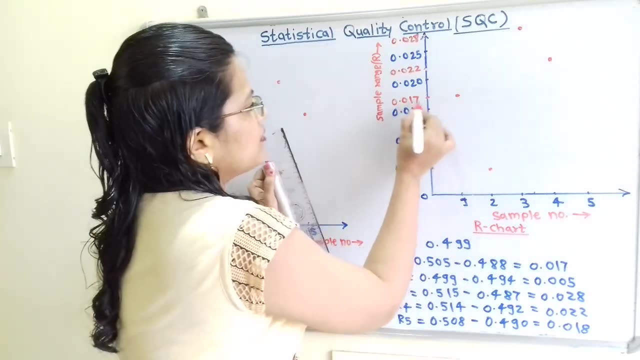 Then here is the point of intersection. So this is our fourth reading. Then for the fifth it is 0.018.. Now if we observe, here is 0.015.. So for 18, I have to take. 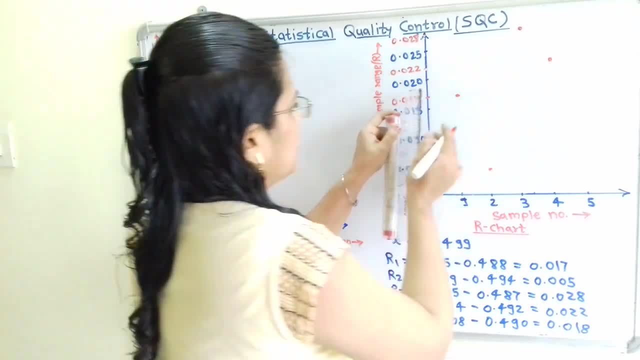 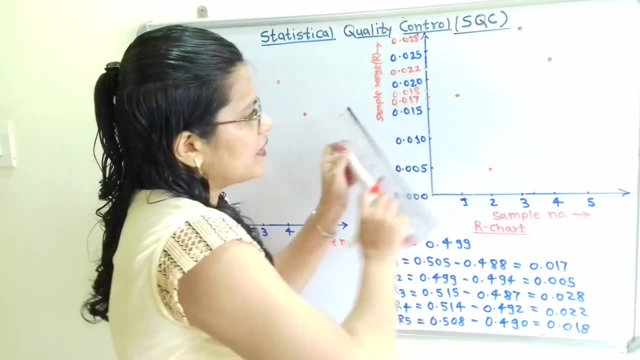 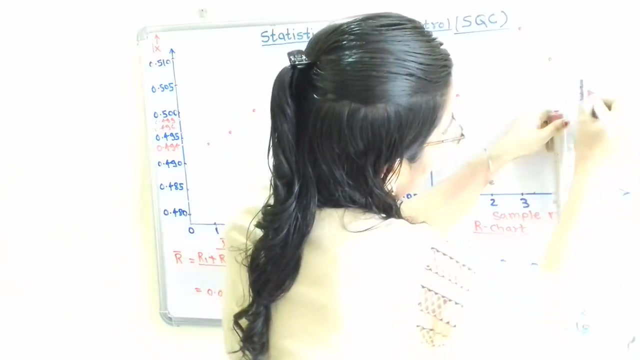 1 centimeter after the 0.017.. So I will mark here 1 point and this will be 0.018.. And if I take here 1 horizontal line, Then here is the point of intersection. So this is our fifth reading. 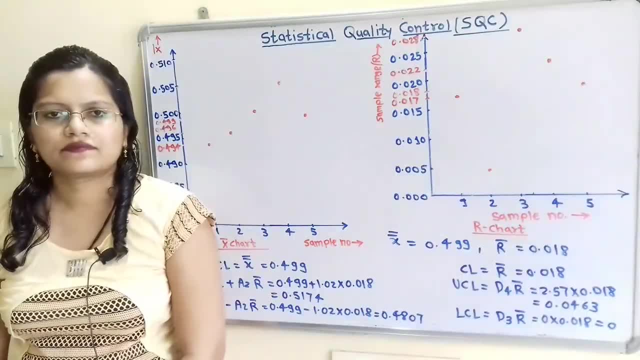 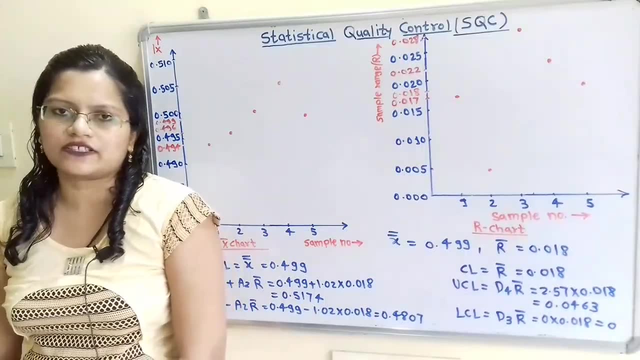 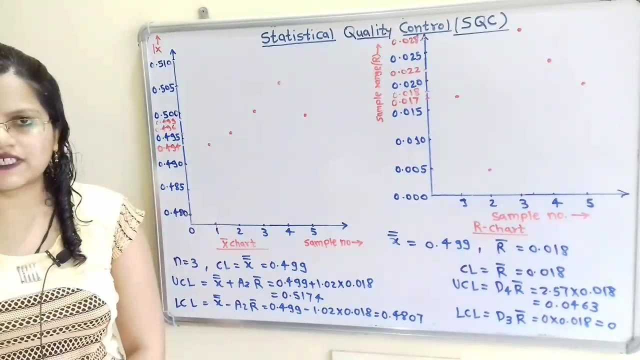 Now we will calculate the control limit values for the X bar chart as well as R chart. Now there are three number of observations. So value of n that is equal to 3.. Now how to calculate this value for the center line. So C L is equal to X bar. So C L is equal. 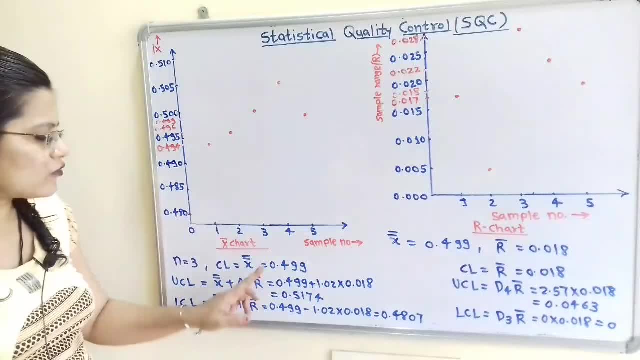 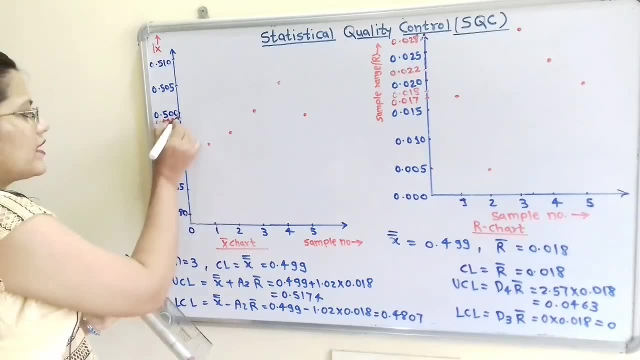 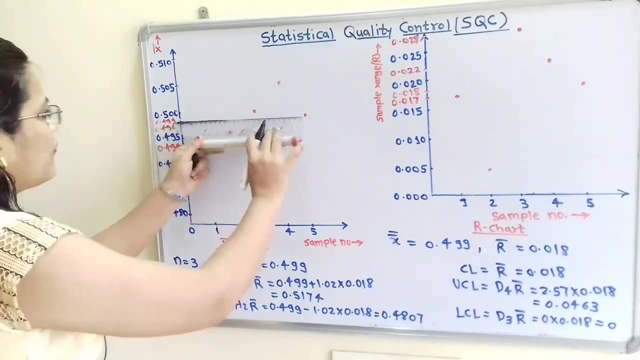 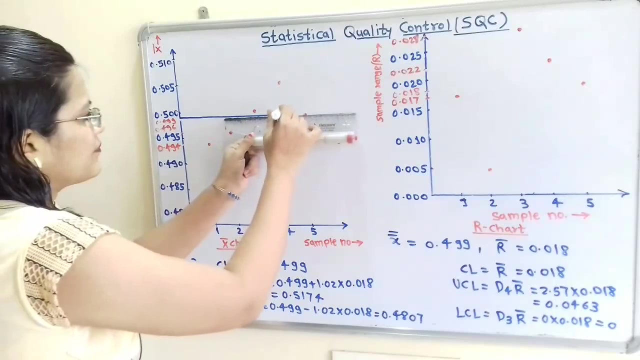 to X double bar And this value, we have already calculated 0.499.. So I have to show here Now, if we observe, here is the point that is 1 centimeter below this: 0.500.. There is 0.499.. So from this I have to take here 1 horizontal line. So this is the value for. 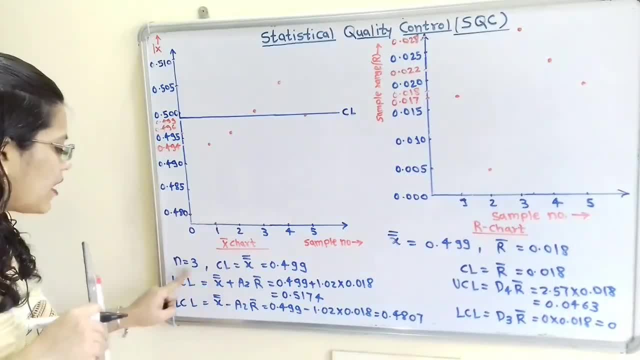 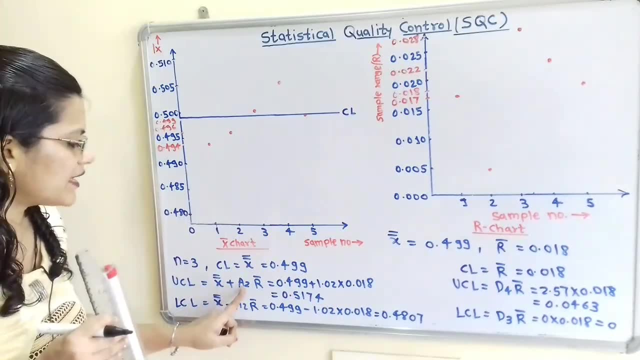 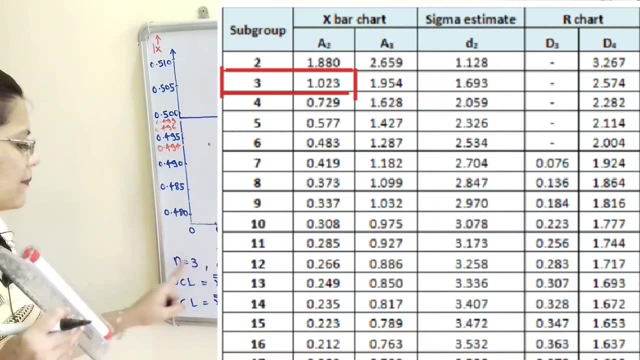 C, L, That is the center line, Then upper control limit. So for this upper control limit formula is X double bar plus A2 R bar. So this value of A2, we have to find out from this sample size. So sample size n is equal to 3.. So if we observe this chart for sample size 3,, 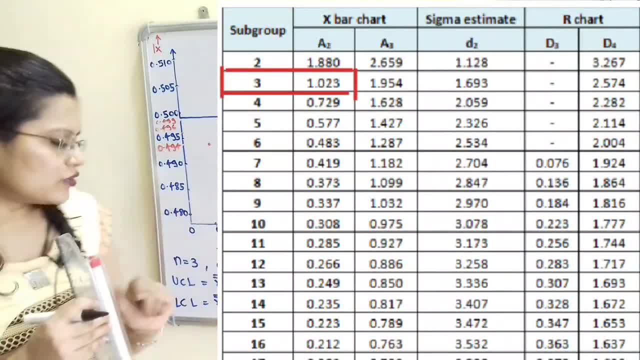 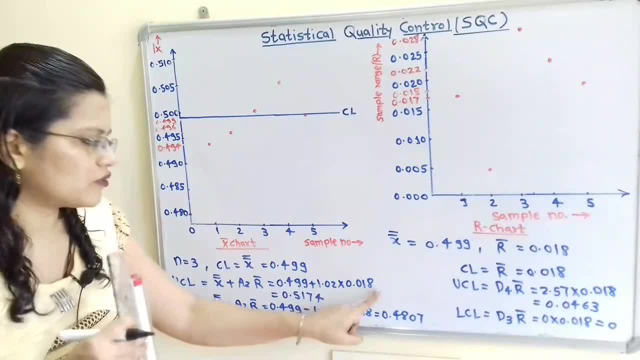 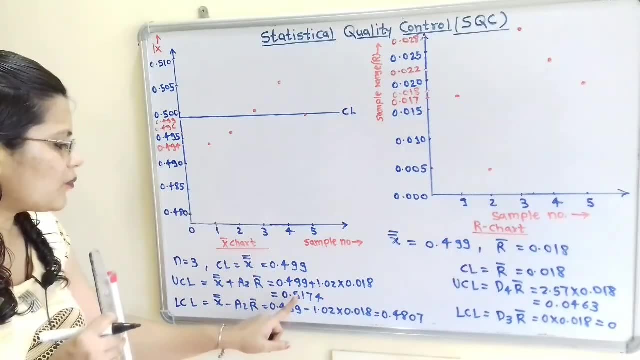 value of A2 is 1.02.. So we will take here 0.499.. And plus 1.02 into 0.018, because R bar is 0.018.. So when we calculate this then we will get the answer 0.5174.. So we have to draw here 1 line. Now, if we observe here: 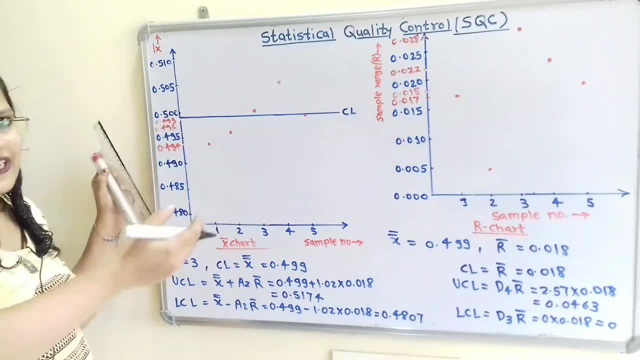 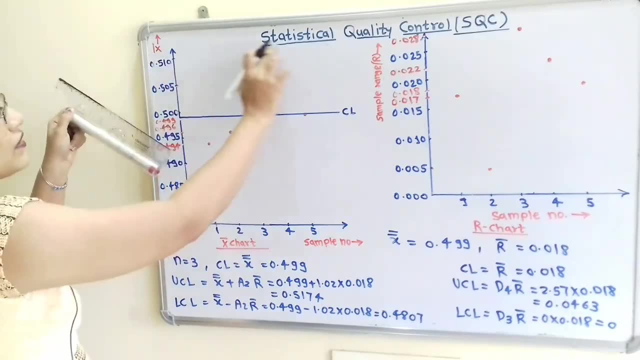 is 0.510.. That is 510.. Then after this 7 centimeter, because of limited space available, I will draw here 1 line, That is for the 0.018.. So I will take 0.5174 because of the limited space, But we have to take here the 7 centimeter. 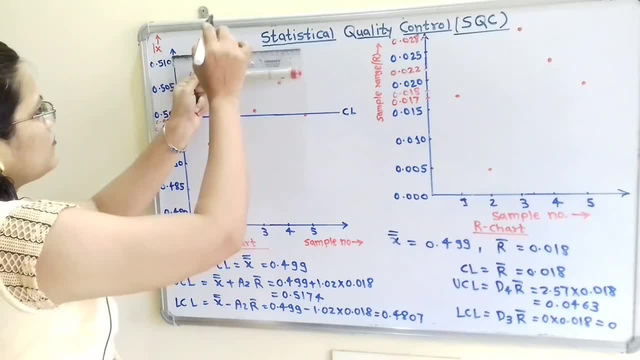 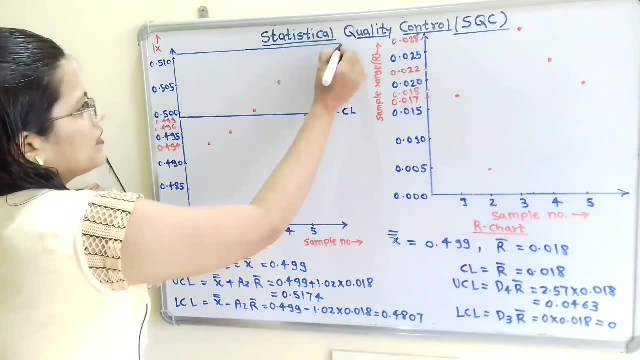 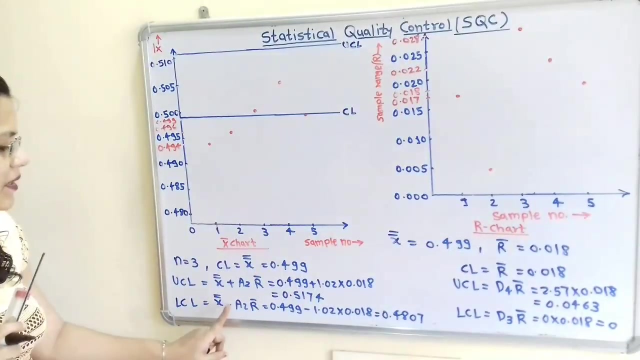 after this 510.. So I will take slightly upward. And here is this upper control limit, That is U C L. Now we will calculate lower control limit And formula is X double bar minus A2, R bar. So this value of A2, that is 1.02.. That means we have to take here 1.02.. So 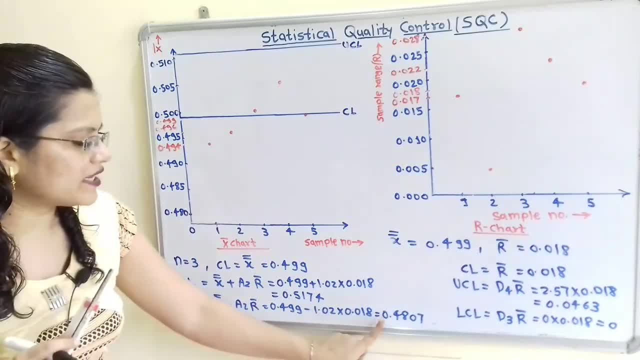 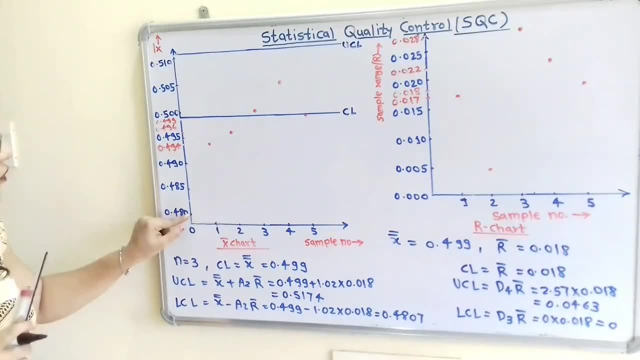 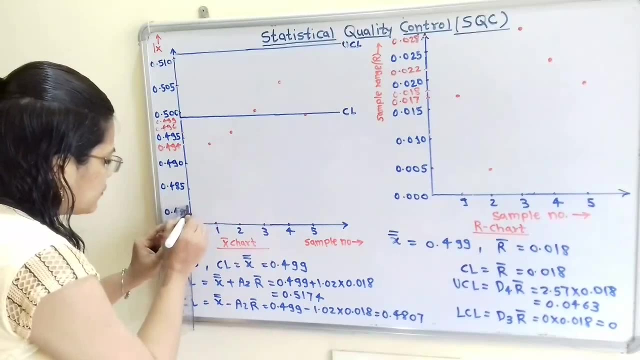 we have to take And if we calculate then we will get the answer 0.4807.. So we will take in between 0.480 to 0.481.. That is because it is after 0, there is 7. So it is nearby. 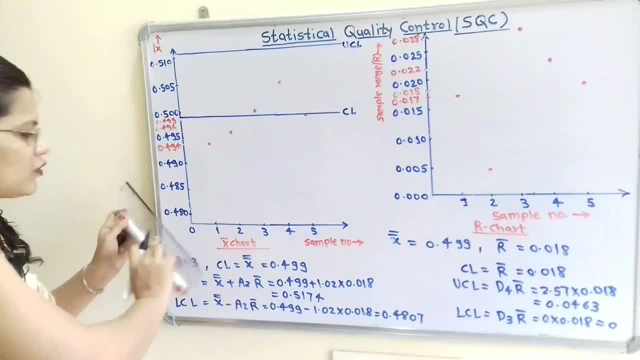 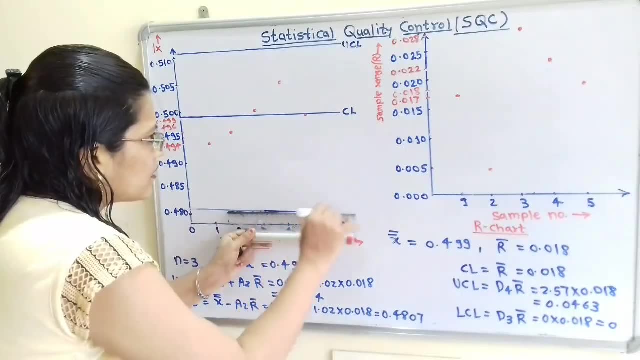 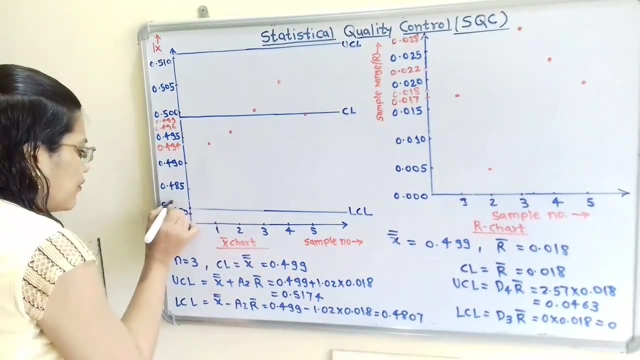 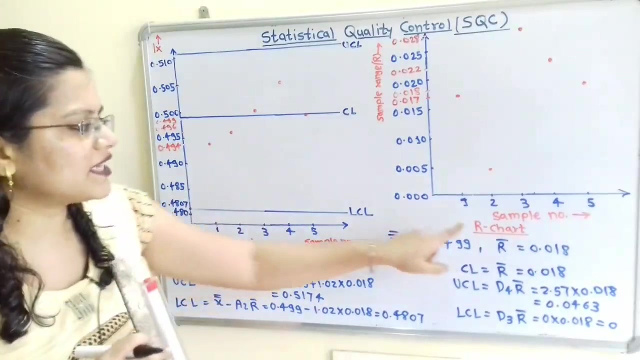 to 0.481.. So I will take here 1 approximate line, And that is for this lower control limit, And the value for this point is 0.4807.. Now we will move to the next chart, That is the. 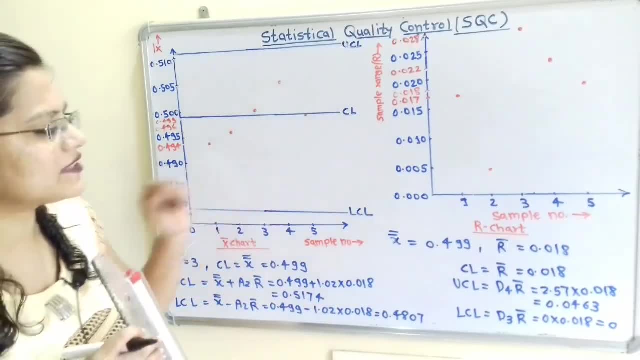 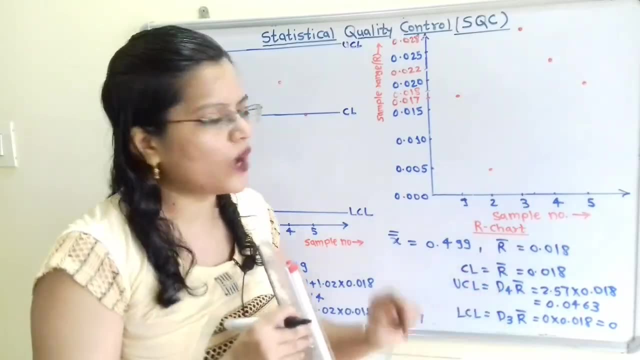 R chart. So for R chart also we have to decide these values. So how to decide the value for the center line? So center line is equal to R bar And that is 0.018.. So how to plot this 0.018?. 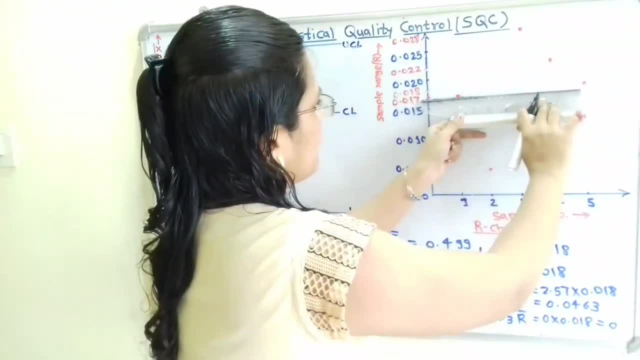 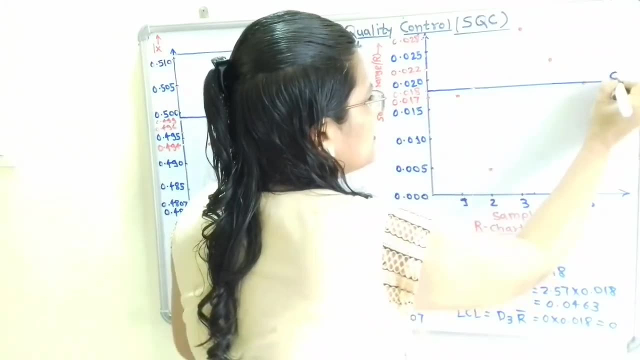 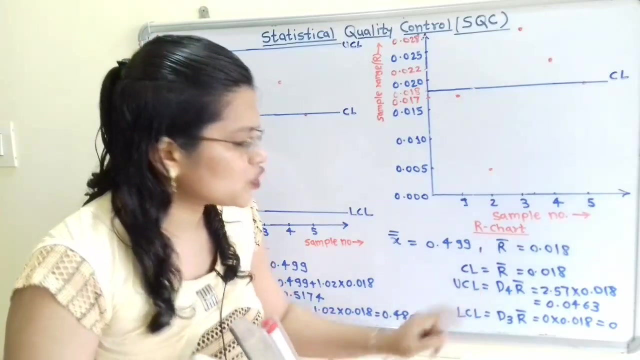 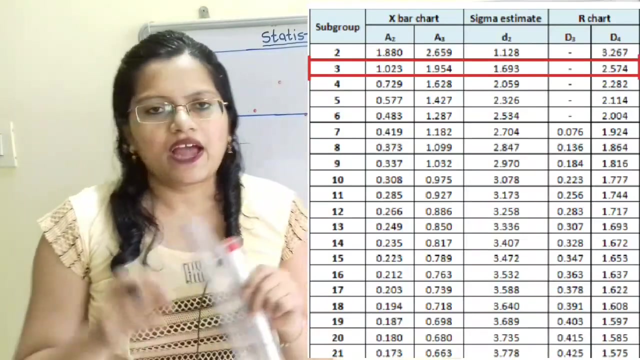 So here is the 0.018.. So we will consider here one line, So this is the center line, Then upper control limit. Now if we observe, for this upper control limit again we have to refer the sample size. So sample size n is equal to 3.. And for this upper control 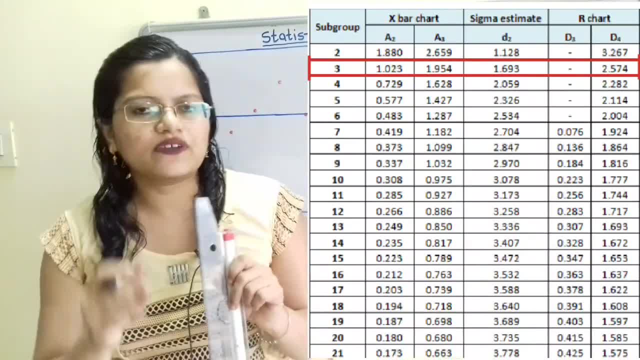 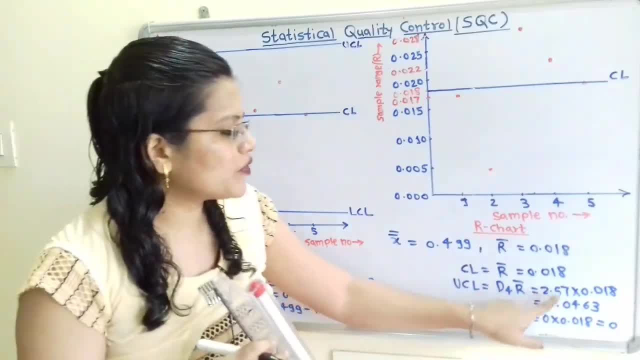 limit, we will refer the value for default. So if we refer the value for default, we will refer the value for default. So if we observe this chart, then value of default is 2.57.. So what is the answer- 2.57 into. 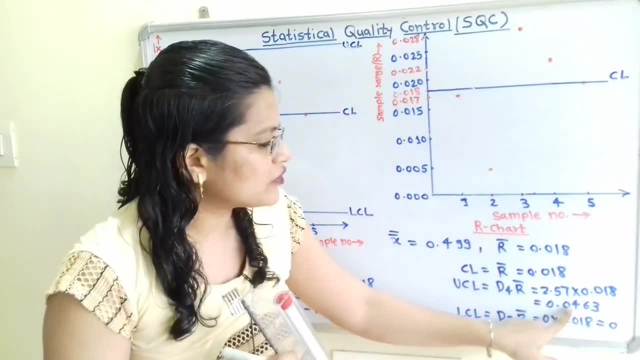 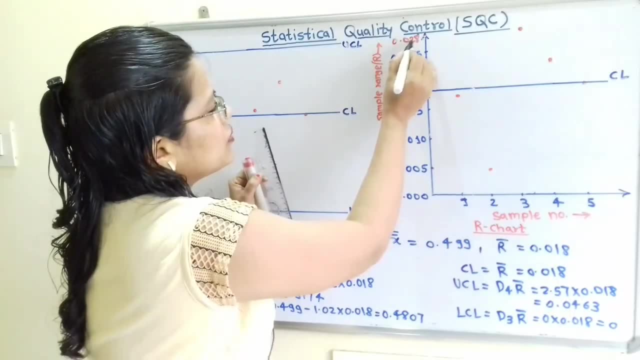 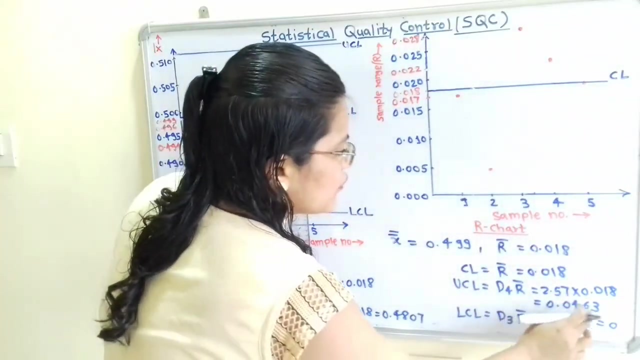 0.018,, which is equal to 0.0463.. Now, if we observe, here is our last value: 0.028.. After that it is 0.030.. And then there is 0.0463.. So, because of limited space available, this: 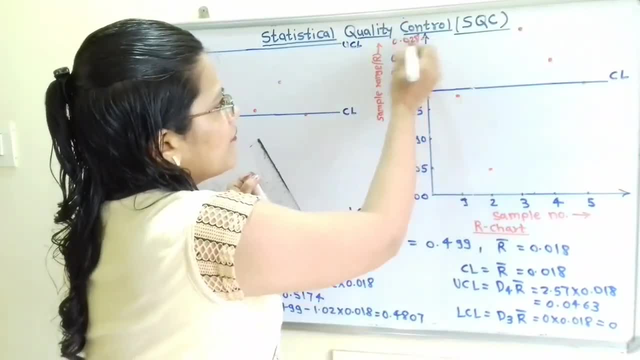 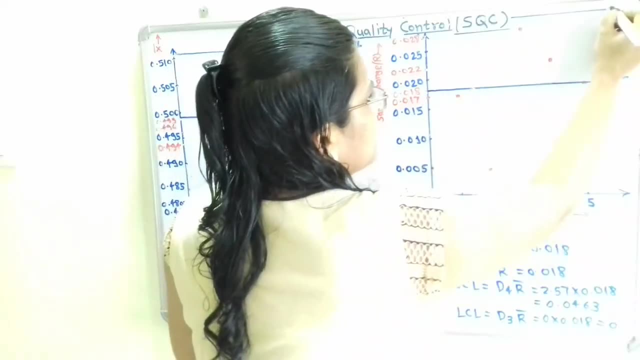 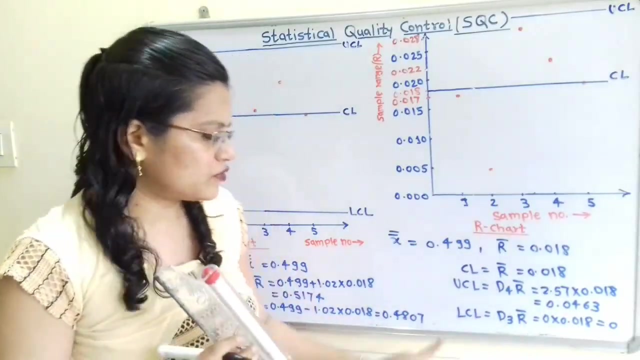 line is much higher than this, our largest point. So I will consider here the approximate line, because of limited space, And this is the upper control limit. Then we will move to calculate lower control limit. So for lower control limit, formula is D3R bar. So